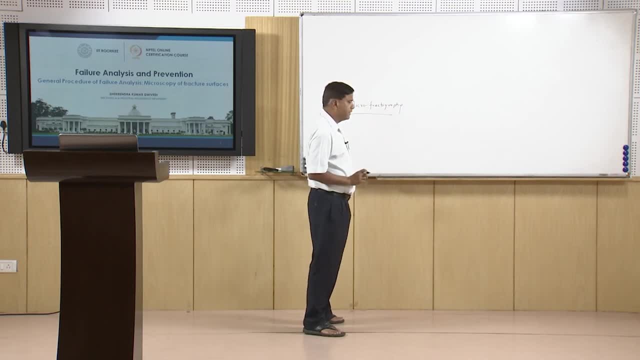 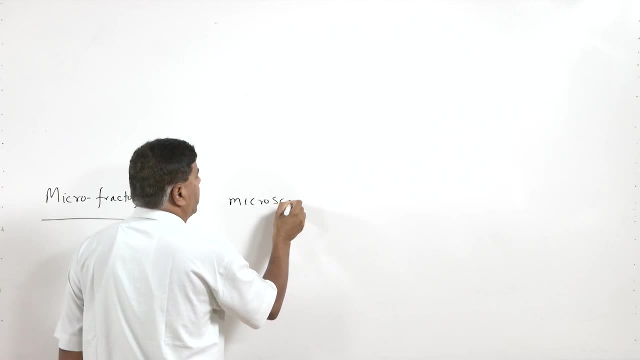 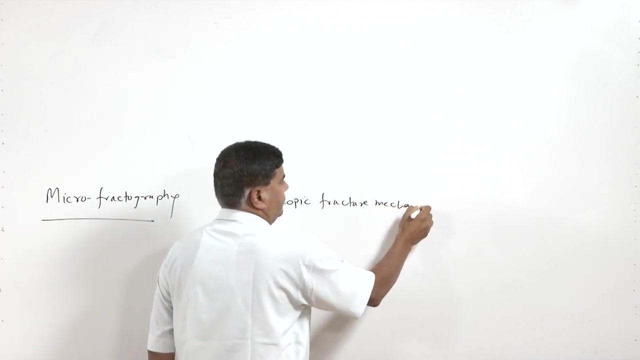 of the fracture surfaces, or we can say microfractography, we try to understand the macroscopic fracture mechanisms. A mechanicalทำ is Where, if the crack which has nucleated how this crack will be growing to facilitate the fracture at a micro level. So basically, this is called and although 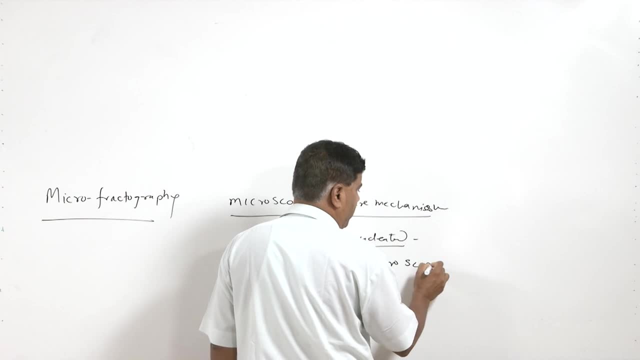 occurs on the surface and get so. basically, this is called microscopic. These are also called microscopic mechanisms of fracturepersons. Never forget about it. so another point where we grow, or if material isанный because we fill this haut, nasıls to posture? we know? 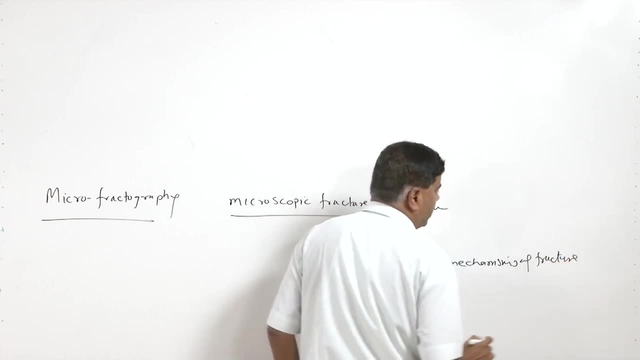 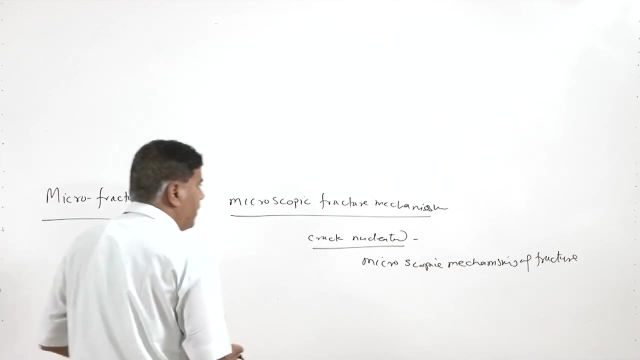 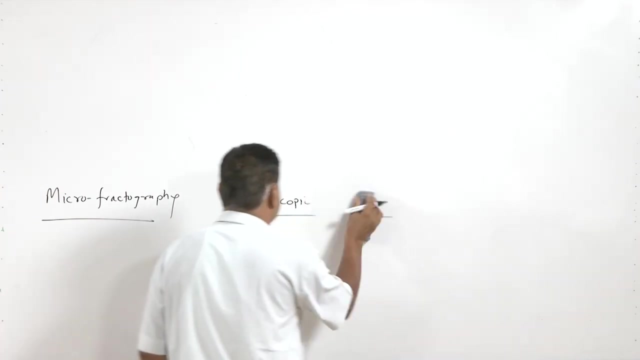 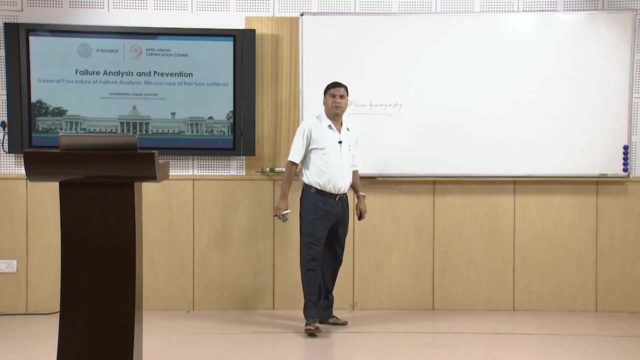 Raymond M want you to understand that in such OD fast this might get into various contains fracture, because the way by which crack grows during the fracture, that is what we try to understand through the microscopy of the fracture mechanisms. There are certain purposes of the microfractography which are achieved through this step, wherein 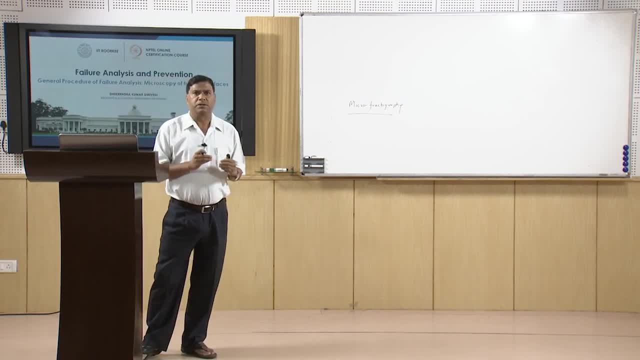 the first one is to identify or to determine the microscopic fracture mechanism which may involve, like the formation of the dimples or cleavage facets, or the intergranular fracture surface or the fatigue striations. So these are the features which will indicate the way by which the crack has propagated. 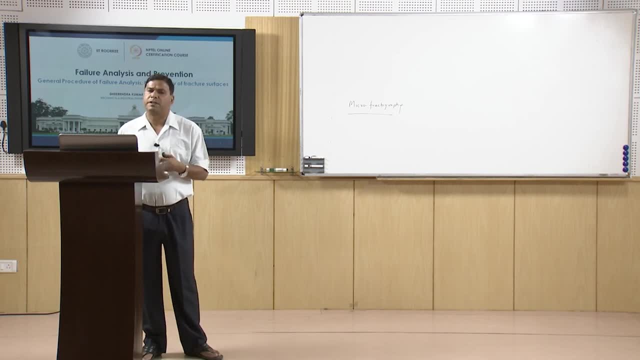 and the kind of the micro fracture. So the one thing is, that which is achieved through the microfractography is the understanding on the microscopic fracture mechanisms, and the second one, it also helps us to understand and classify the fracture in better way, which means there are, like we have, the ductile fracture. 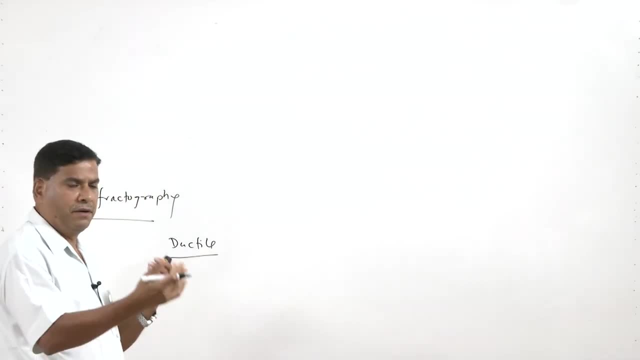 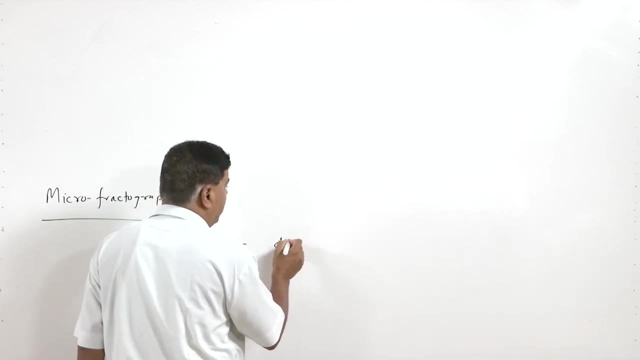 where significant plastic deformation prior to the fracture takes place. Such kind of the fracture frequently occur with the formation of the dimples on to the fracture surface. So one the feature which is generally obtained in case of the ductile fractures which involve lot of plastic deformation prior to the fracture, is the formation of the dimples, which is nothing. 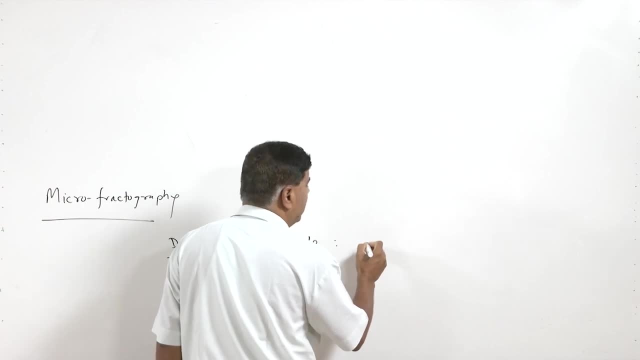 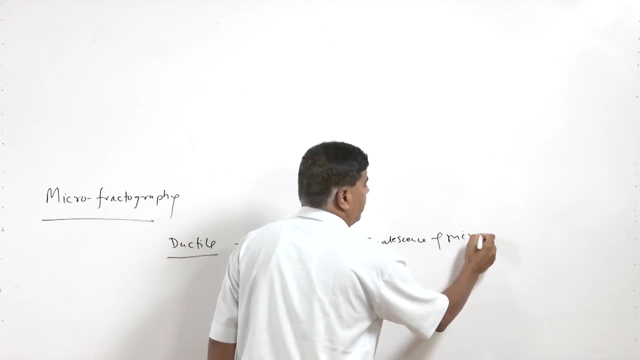 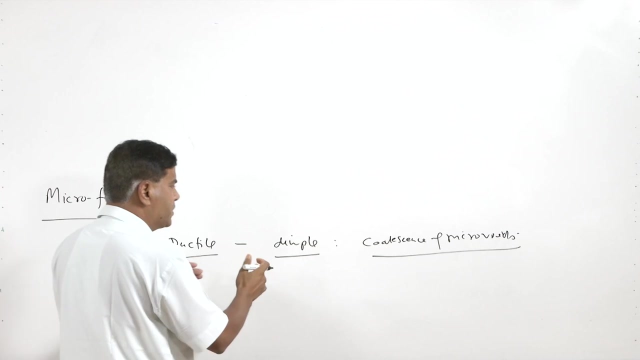 just, it is about the coalescence of the micro voids which are nucleating. So whenever this mechanism is involved then it leads to the development of the dimples on the fracture mechanism and this leads to the ductile fracture means the. this is very 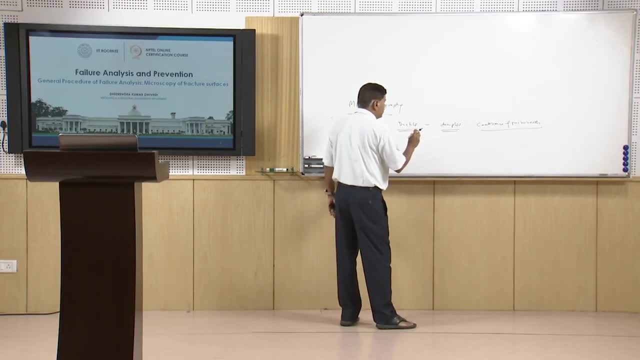 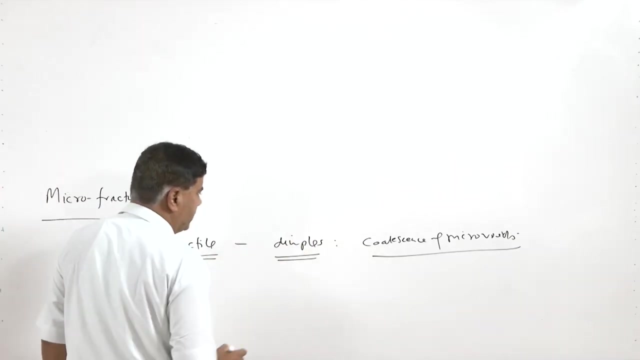 general one. So there can be in some of the specialized cases where the fracture is brittle, means there is no plastic deformation, major plastic deformation, but still we see the dimples. But in general the ductile fracture are accompanied with the brutal fracture. 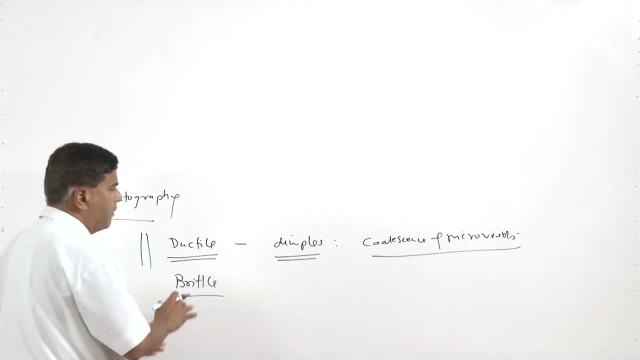 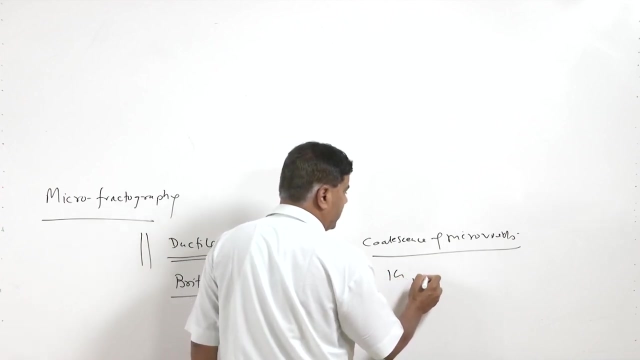 Similarly it also helps, like in brutal fracture. the fracture may occur through the different the fracture surface features, like the cleavage facets. So that's all, Thank you. cleavage facets, or there can be intergranular fracture or there can be the presence of. 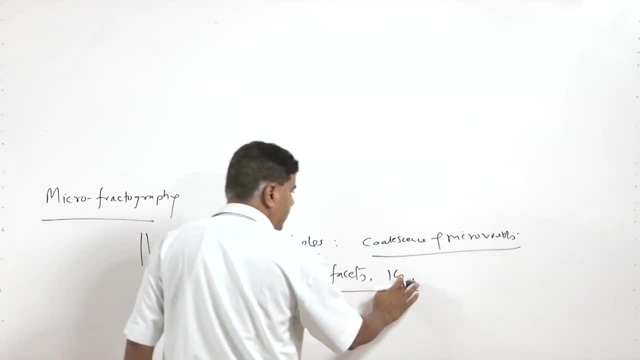 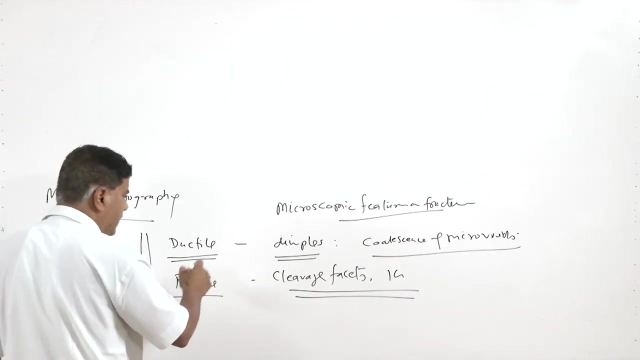 so these are the two features which will be involving the brittle fracture and so these can be observed only at a higher magnification and that is why we call it as a microscopic features of the features on fracture surfaces. So these are the two broad grouping to understand, similarly, if there are many other, the ways 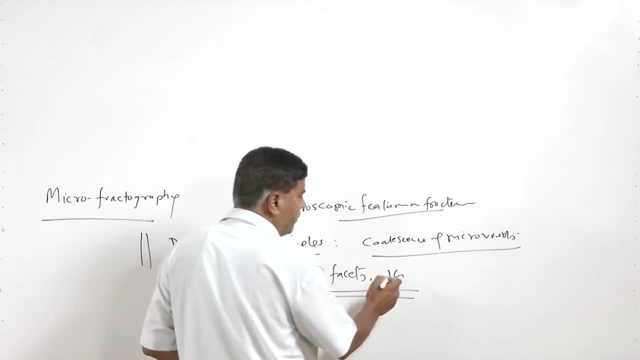 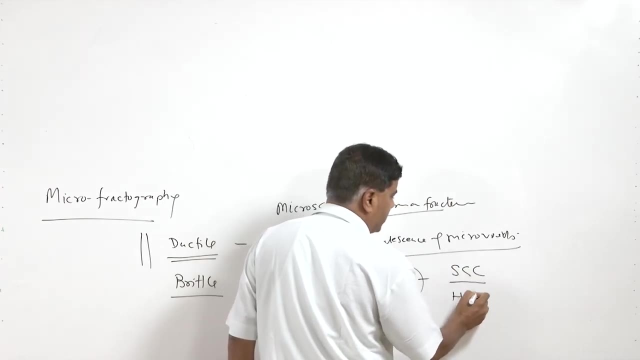 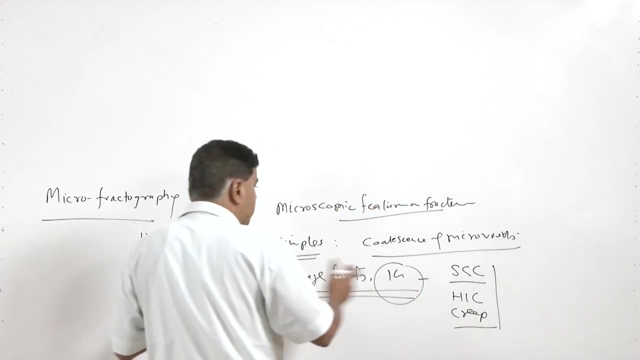 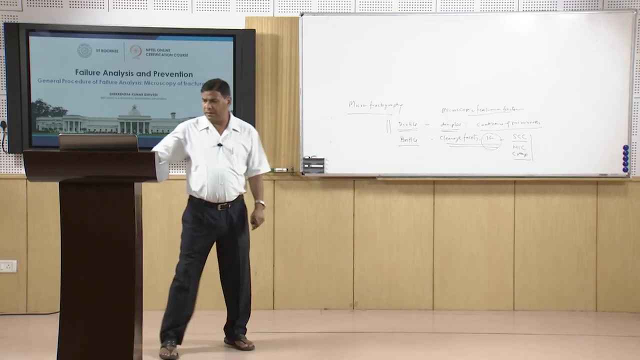 by which the intergranular fracture can take place. like it, there can be involvement of the stress, corrosion cracking. there can be the hydrogen induced cracking. there can be the cream, There can be fracture, but these can be substantiated only through the microscopic fracture mechanisms. 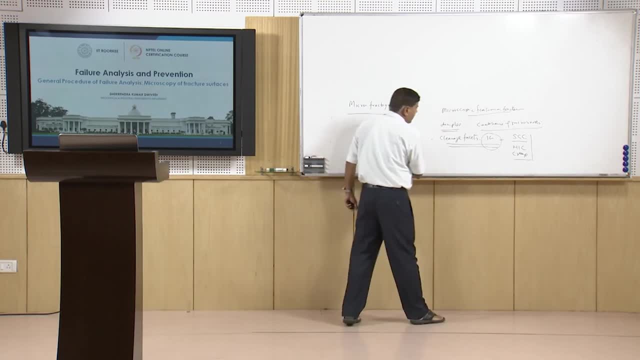 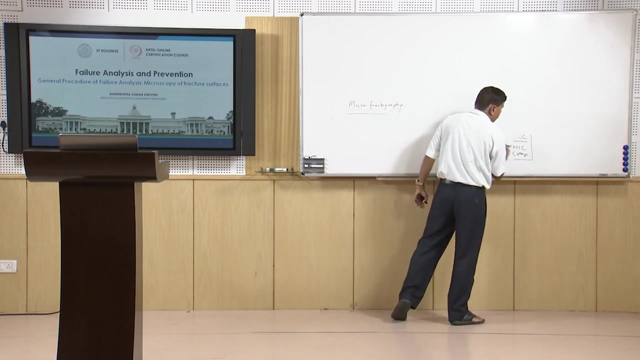 So means the microscopy of the fracture surface helps in identifying these features present on the fracture surface, which will indicate the possibility of the ductile or the brittle fractures. So there can be some of the. however, there can be some of the exceptions, where the just 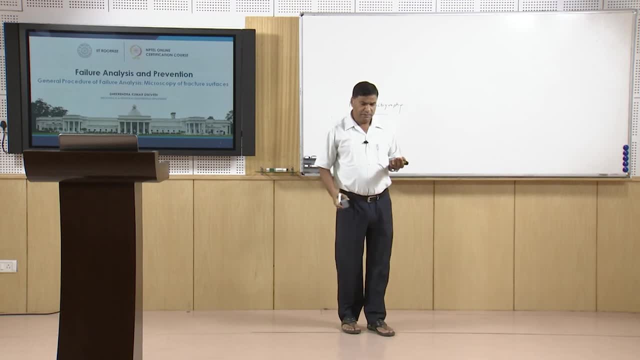 opposite situation. maybe there like low carbon steel which shows lot of plastic deformation prior to the fracture, but it may all indicate the cleavage presence of the cleavage facets in the steel. So what is this? How much? But neither we find 100 percent dimple fracture. mostly we find the mixed mode of fracture. 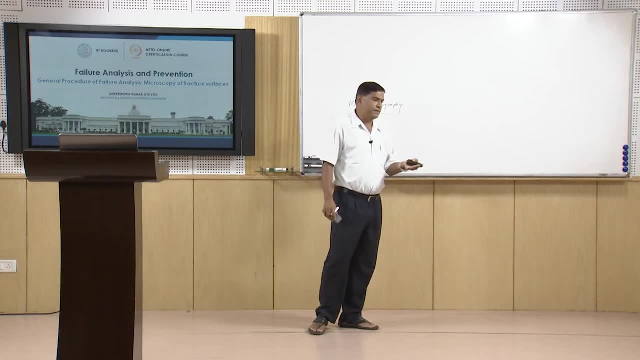 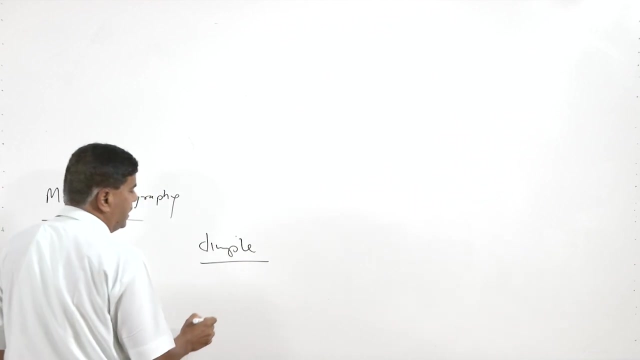 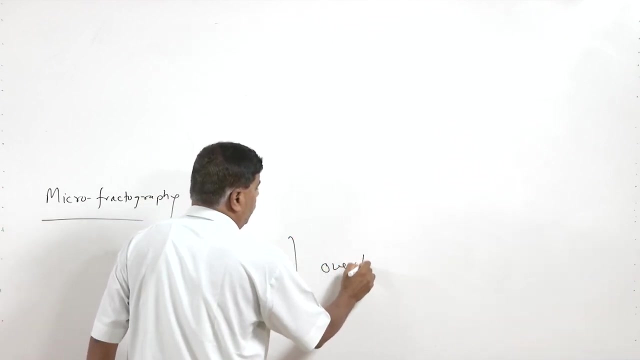 where the presence of dimple and coupled with the cleavage facets are present. so that will be indicating the existence of the mixed mode of fracture. Then estimation of the service condition is the another thing. mostly, like the dimple fracture and cleavage facets, indicates the over load fracture, while the presence of the striations 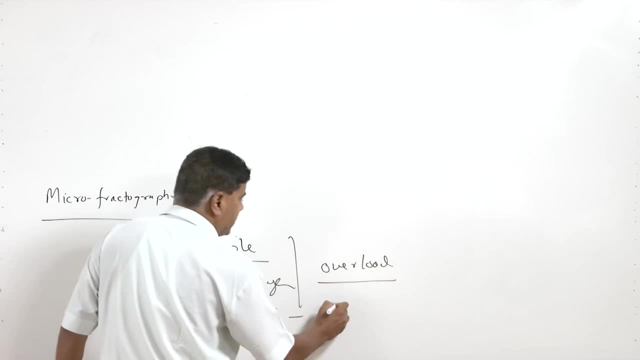 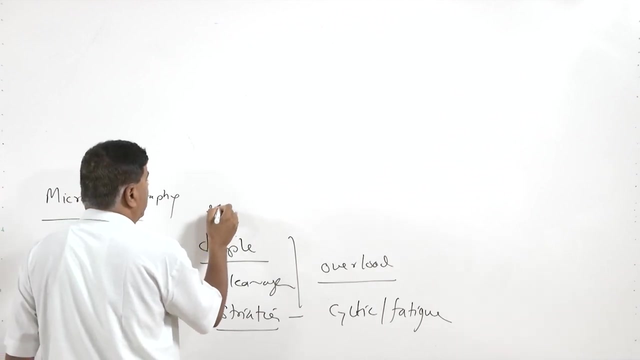 on the fracture surface indicates the cyclic loading or the fatigue fracture. Similarly, the presence of the like, say, inter-gauge fracture, Granular fracture, inter-granular fracture- where the grain boundaries have been eaten out by the corrosion, indicating the stress corrosion cracking or stress corrosion cracking. 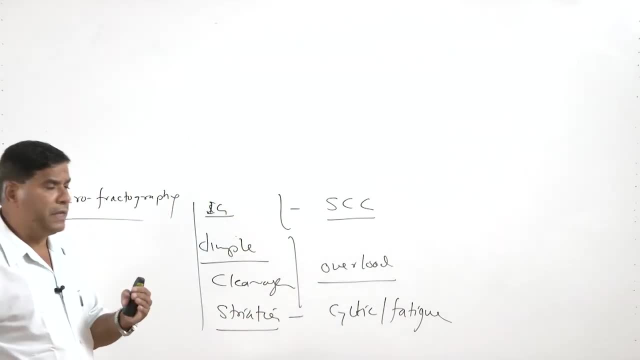 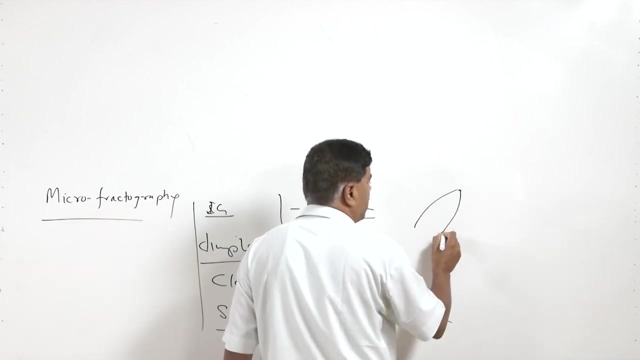 So these are the basically the features which will indicate the load, the type of load under which failure has taken place or the conditions in which a fracture has taken place. Likewise, if the dimples are elongated in particular direction, then that can indicate. 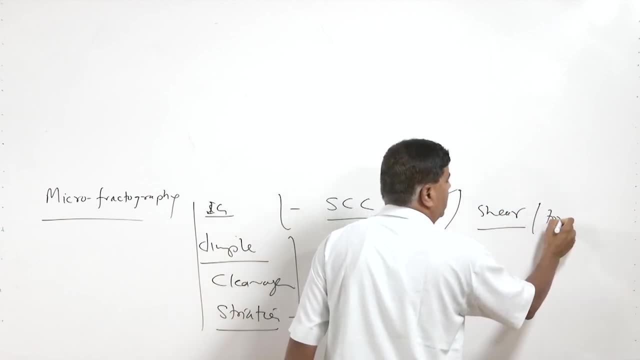 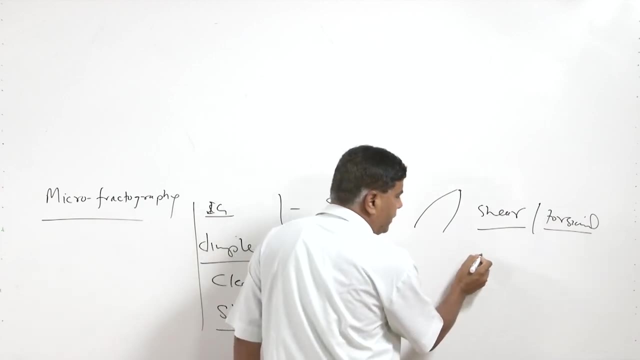 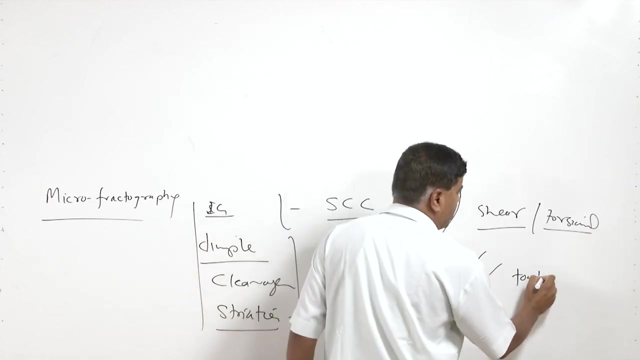 the possibility of the shear or the torsional loading. This kind of the features are also observed where the dimples are oriented in one particular direction on the fracture surface. So that happens especially in case of the toughness test where component surface is subjected to the shear. 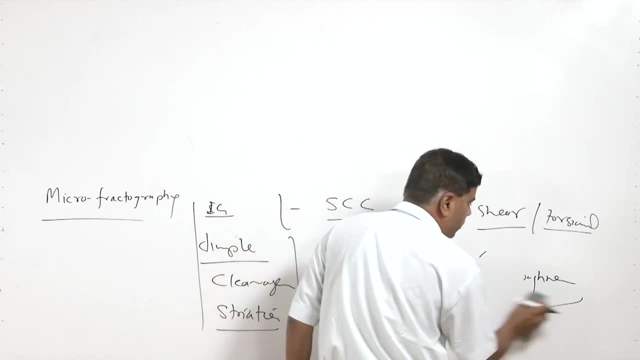 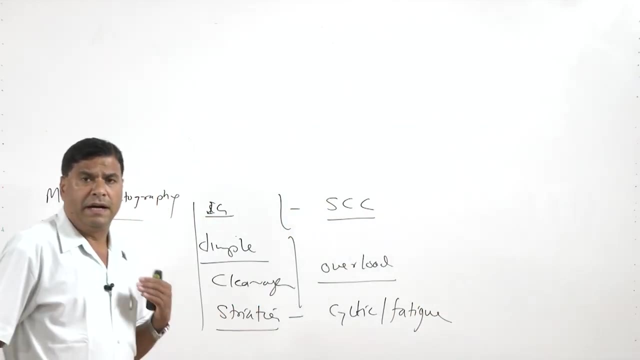 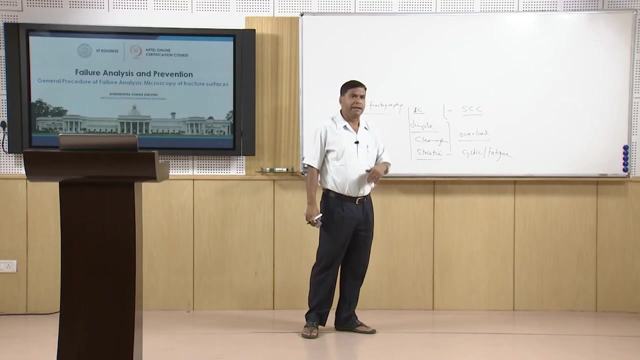 So the kind of the load which has acted on to the under which the failure has taken place can also be identified through the microfractography. So the type of load, whether it is over load, cyclic loading, or the failure has, or it is the shear load or the torsional load, that can be identified through the fracture surface. 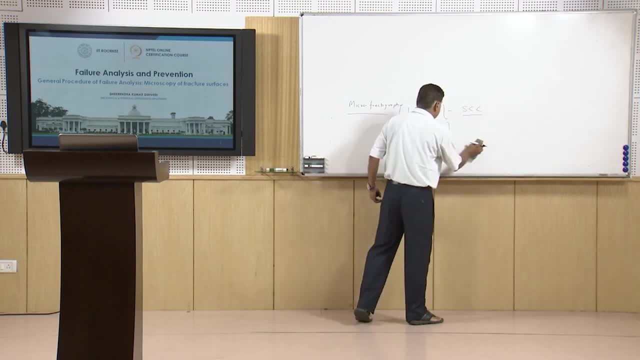 So this kind of the load which has acted on to the under which the failure has taken place can also be identified. So this kind of the load which has acted on to the under which the failure has taken place can also be identified through these microscopic features present on to the fracture surface. 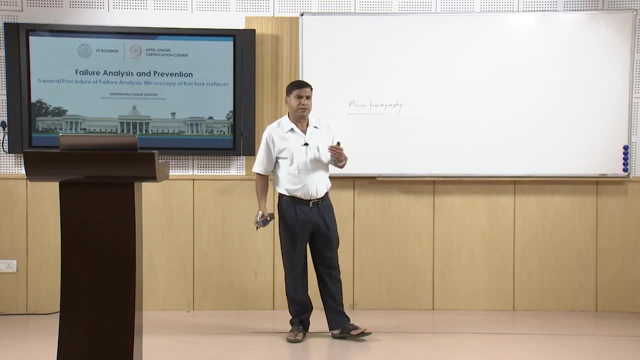 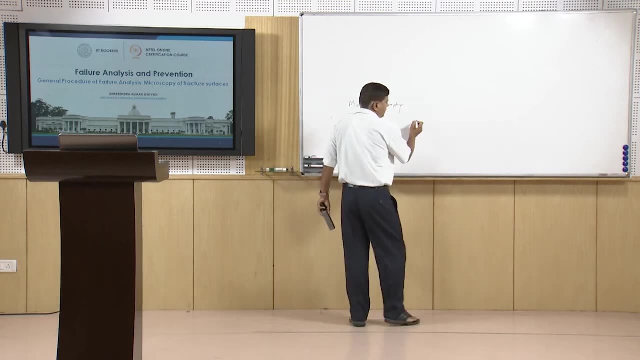 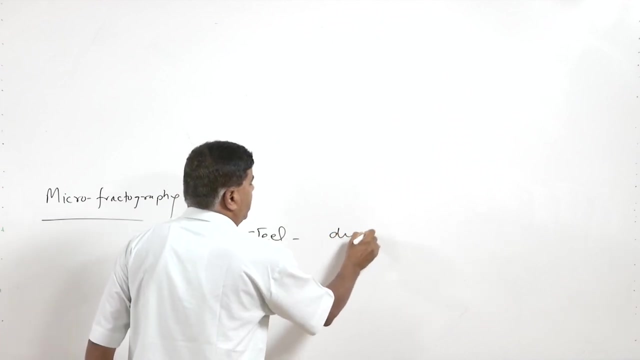 Then sometimes inappropriate. the heat treatment also causes the fracture of the particular kind. like a simple carbon steel normally shows the presence of the dimples on the fracture surface indicating the ductile fracture. So this kind of the load which has acted on to the fracture surface can also be identified. 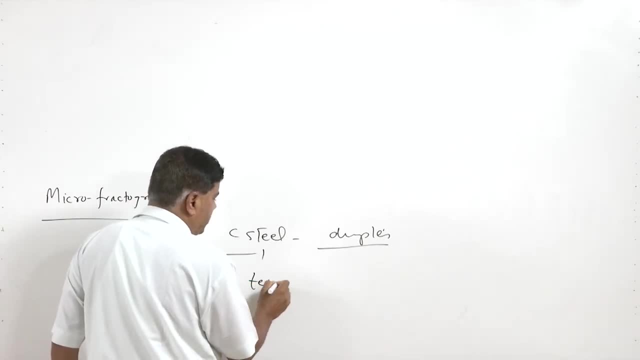 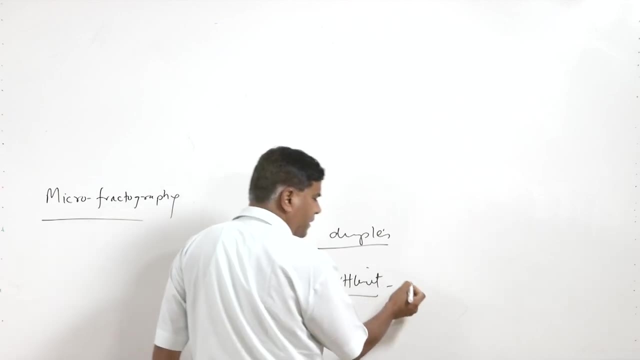 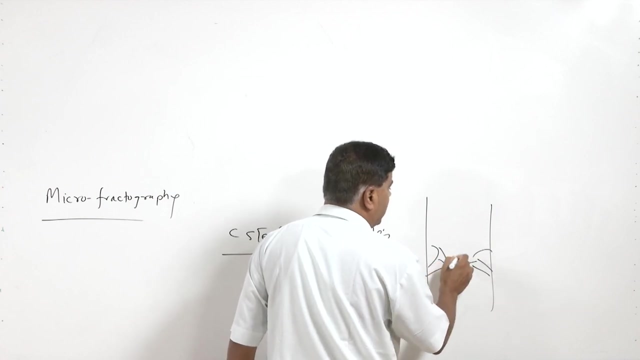 through the microfractography. But if the same steel is subjected to the heat treatment in temper embrittlement range, then temper embrittlement causes the precipitation of the certain unfavorable constituents at the grain boundaries and that in turn leads to the intergranular fracture. 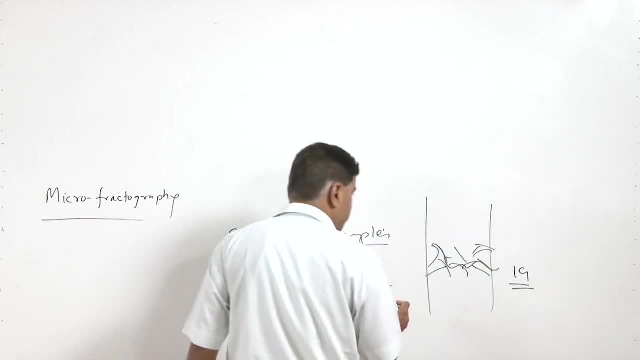 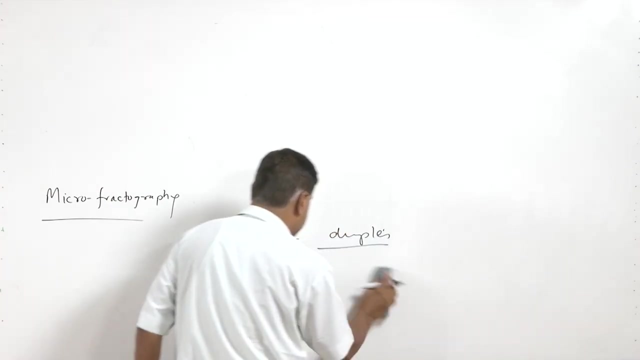 So intergranular fracture can also occur in the steel if it has been subjected to the improper heat treatment. Similarly, there are various types of heat treatment. Similarly there are variety of the alloys and the metals which if are given in appropriate environmental conditions at elevated temperature, then they show embrittlement and that happens. 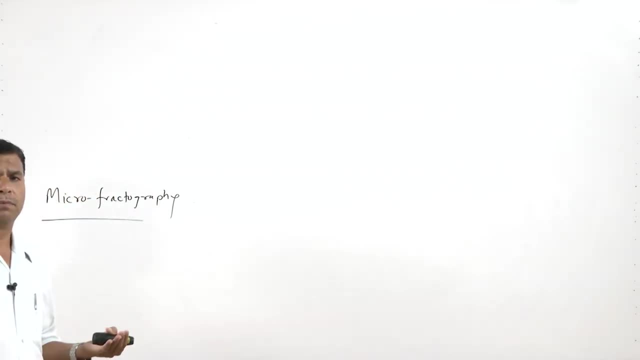 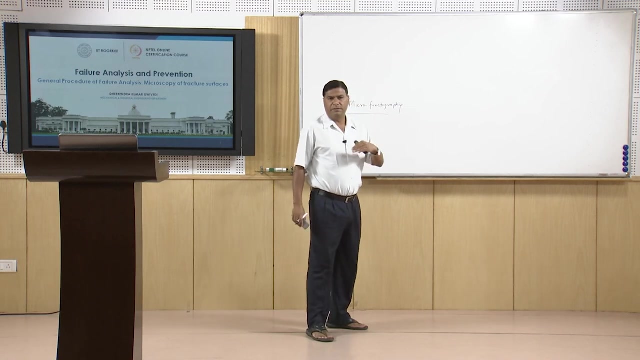 primarily due to the inappropriate manufacturing condition, and this kind of the failures may occur in form of the intergranular fracture. So this kind of the failures may occur in form of the intergranular fracture. Similarly, there are variety of the alloys and the metals which, if are given in appropriate 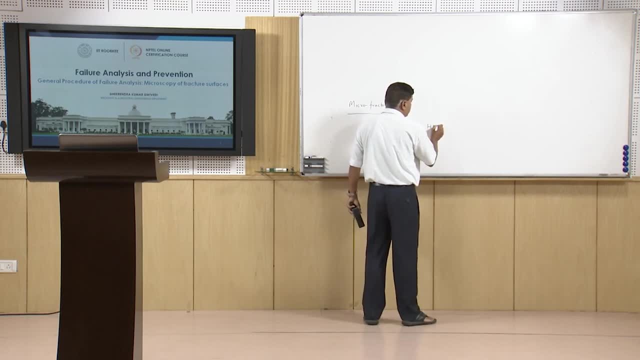 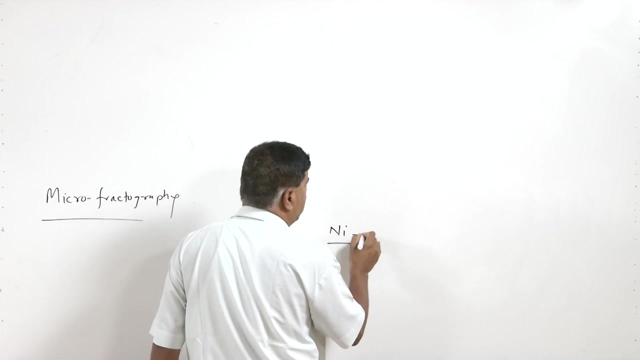 environmental conditions and this kind of the failures may occur in form of the intergranular fracture, So the hydrogen induced cracking or the temper embrittlement or the precipitation of the undesirable things, like in super alloys, or in super alloys like incunal presence of the 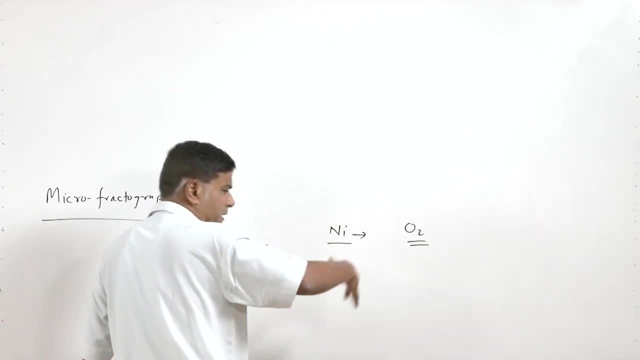 oxygen at the grain boundaries can lead to the embrittlement of these, So hydrogen in case of the steels, Oxygen in case of the steel. Oxygen, Oxygen, Oxygen, Oxygen, So the nickel alloys. in likewise presence of certain specific elements at the grain. 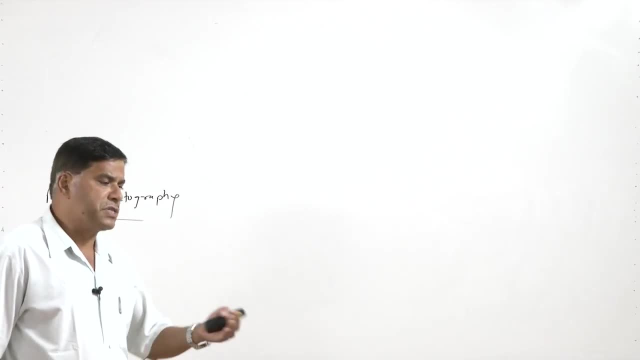 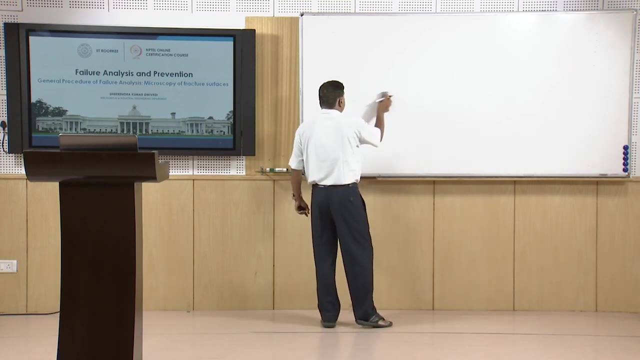 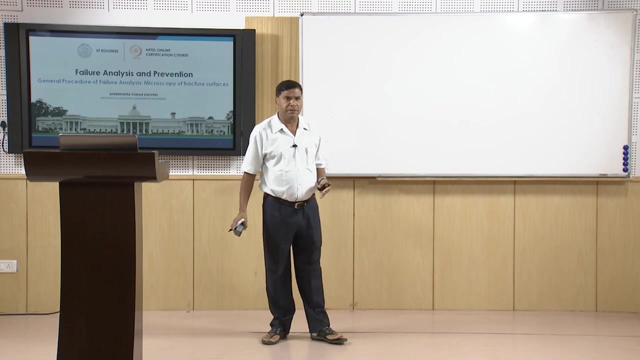 boundary due to the unfavorable manufacturing conditions, can lead to the intergranular fracture. So the purpose of the microfractography is to understand the microscopic fracture mechanism, to classify the fracture in better way and to estimate the possible service conditions in terms of the load and the kind of unique environment. 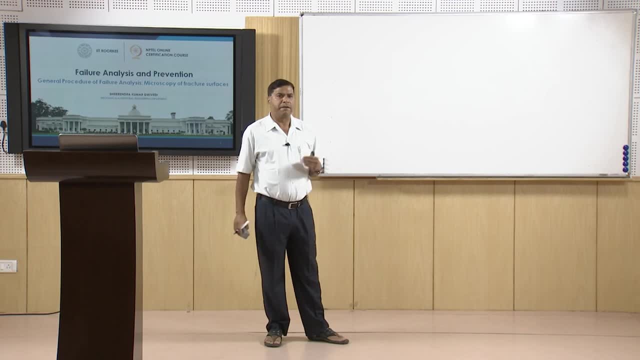 Like corrosion or oxidation, and then if the component has been subjected to the inappropriate manufacturing conditions where in the precipitation of the certain components at the grain boundary has led to the intergranular fracture. So those things can be estimated through the microfractography. 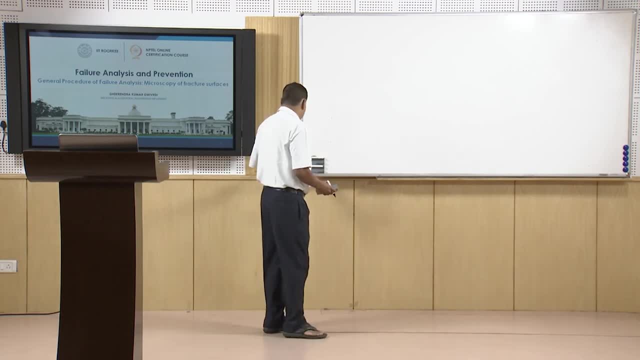 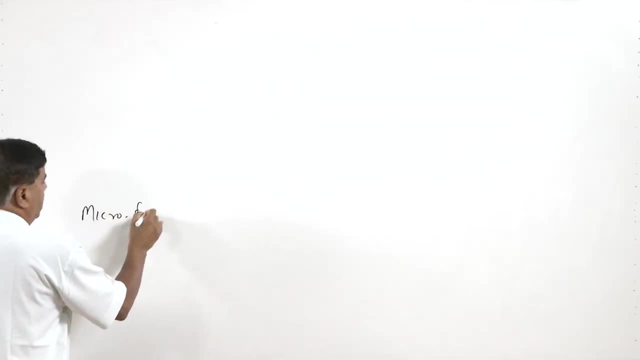 Now how to conduct the microfractography. This is the another aspect. So for microfractography, basically there are, There are two ways which are commonly used. one is the optical microscopy and another is electron microscopy, where in transmission electron microscopy or the scanning electron, 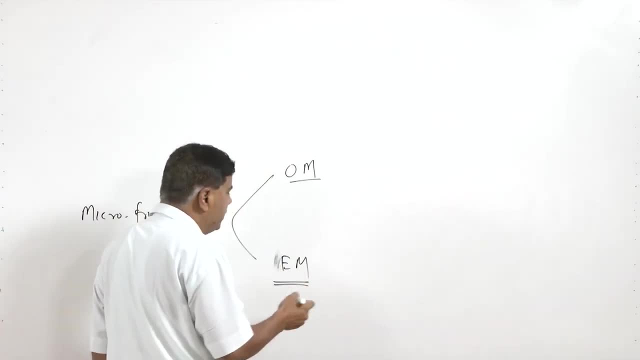 microscopy. both these can be used. It is common or it is preferred to use the scanning electron microscopy, also known as SAM. for scanning electron microscopy, The refractography of the surface- and this is because of the certain regions like it- allows very high resolution, which is the ability to identify the two close constituents clearly. 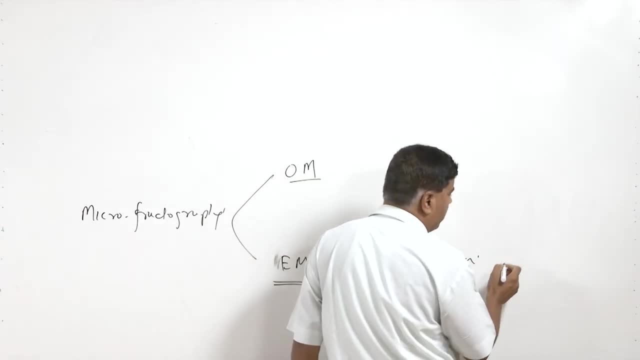 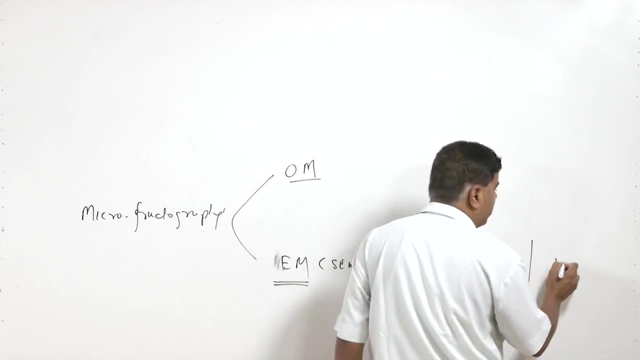 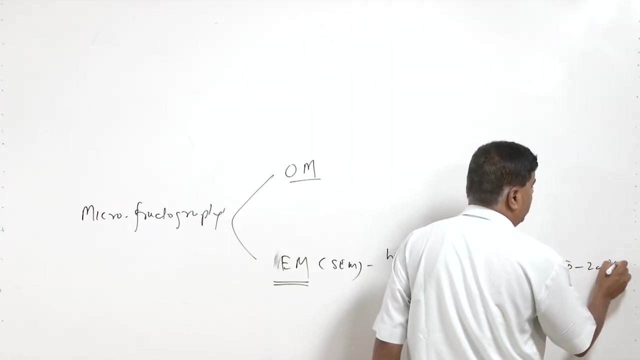 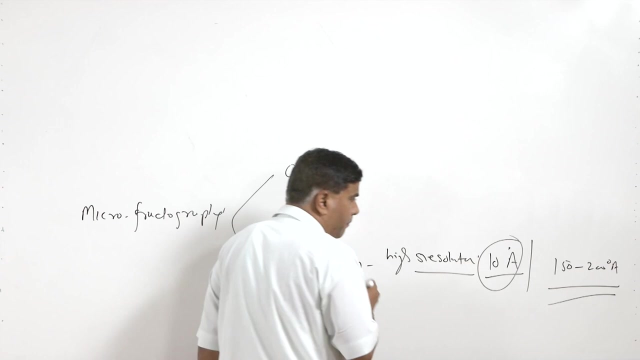 and in case of the TAM or SAM, the resolution can be as low as 10 angstrom, But it is common to have the resolution in these systems of 150 to the 200 angstrom. So this is the minimum side, which is which can be resolved, and the magnification also. 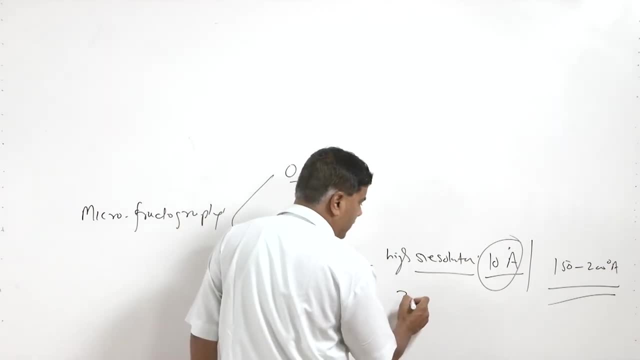 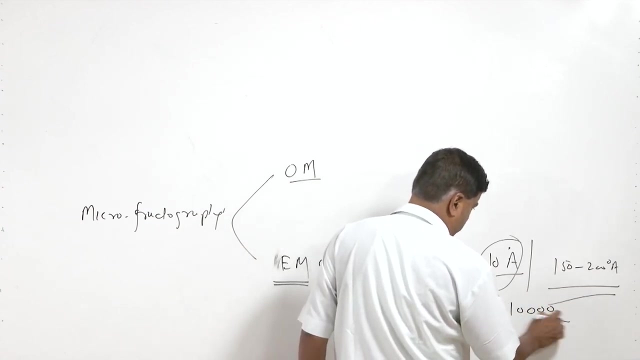 very high magnifications are possible which can go as high as 3 lakhs of the times of the component, the constituents. So 3 lakh magnification is possible But for a failure analysis it is common. like up to 10,000 magnifications are commonly used. 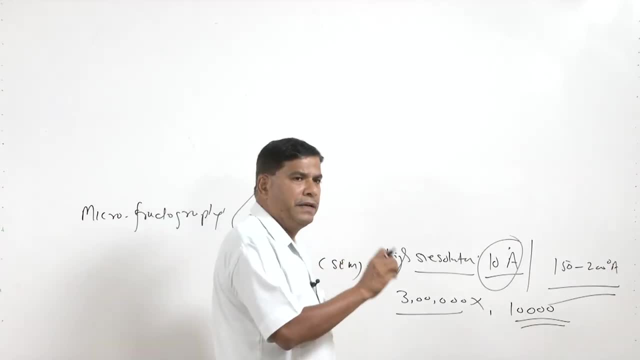 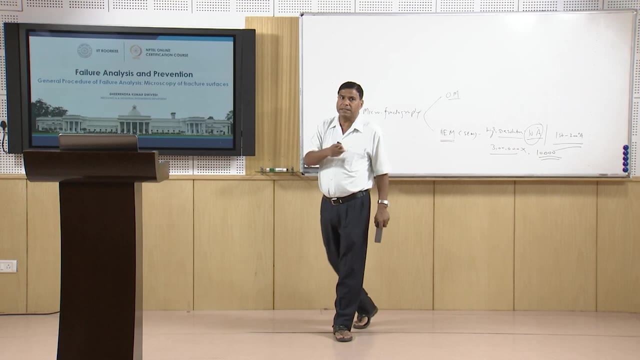 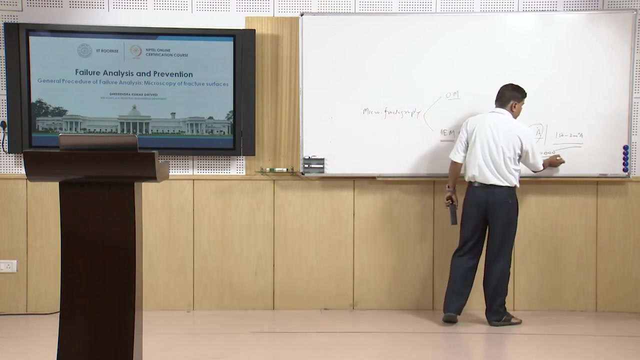 because, above which, we are not able to find any useful information with regard to the refractography, whether it is a precipitation of some fine precipitates at the grain boundary, leading to the embrittlement and cause the intergranular fracture, or the identification of the microscopic fracture mechanisms like the striations. 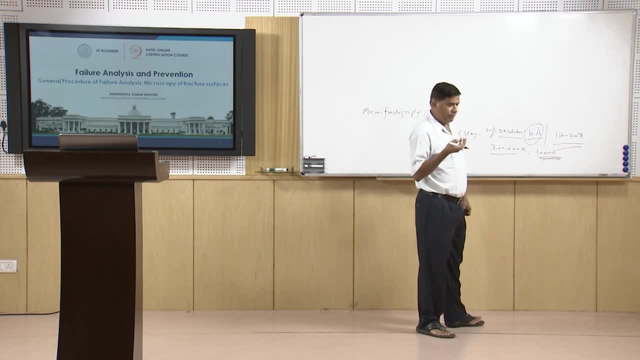 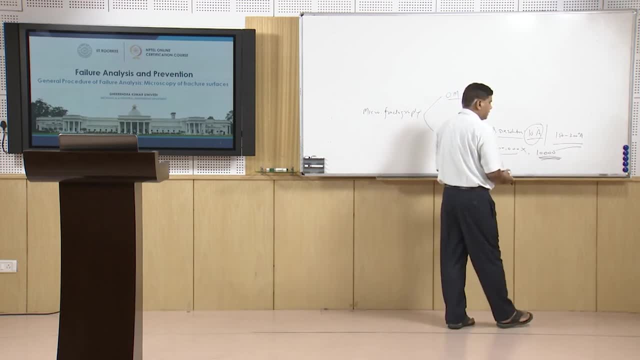 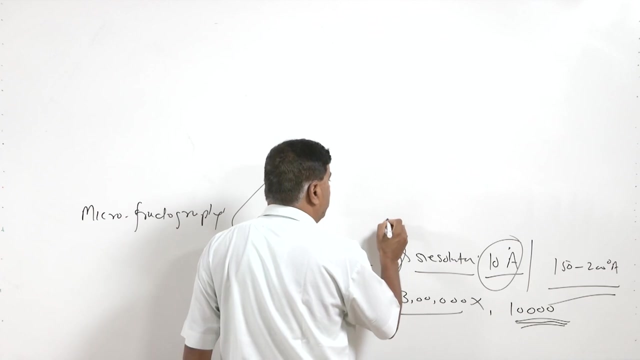 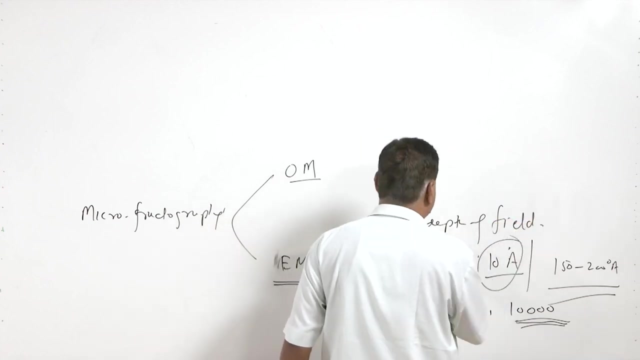 So this is the main reason why we are using this: The intergranular fracture or the cleavage facets or the dimples which are present on the fracture surface, and one more thing, that these do not require any surface preparation. So it is very good that they offer very high depth of field means: the constituents which 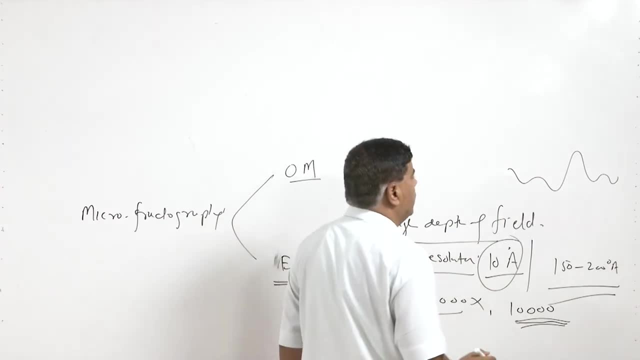 are present. fracture surfaces are obviously rough, So if the depth of field is very high, then all the microscopic features, whatever they are present on the fracture surface, all these can be seen very clearly with the clarity and the presence of the features which are there can be easily recorded. 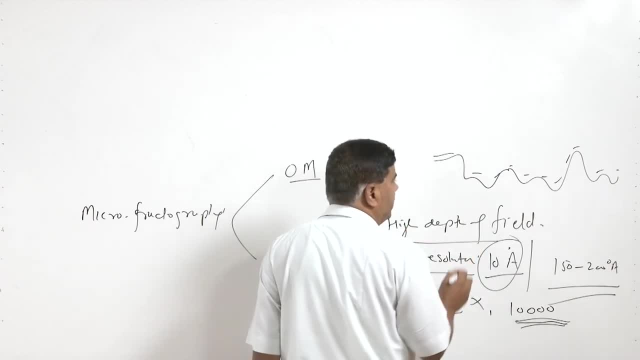 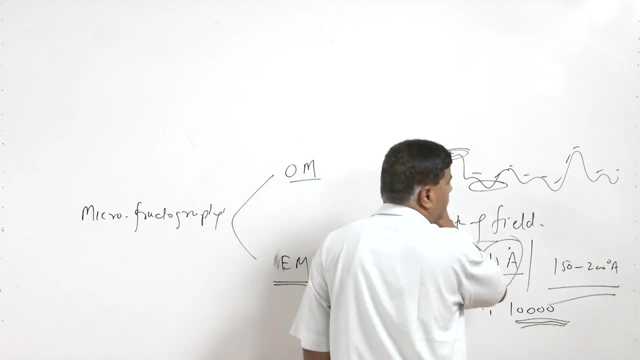 So high depth of field. otherwise, if the depth of field is limited, then this may be good in focus, but other regions may not be. so uniformity in focus will not be good. Somewhere you will find that the one region is in focus and another region is out of focus. 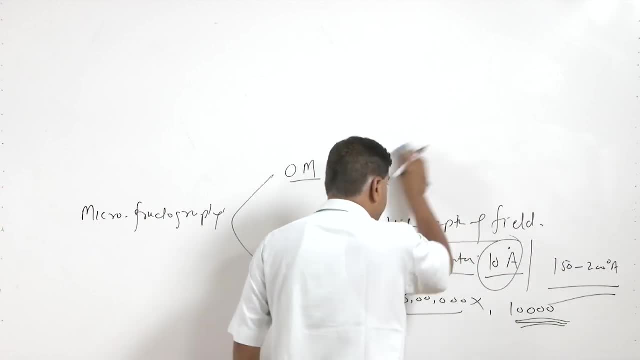 So it is good to have the high depth of field so that the entire fracture surface can be clearly seen. So these are the three aspects related with the SAM, or electron microscopy, Then optical microscopy. here this is normally limited, although we have microscopes of higher. 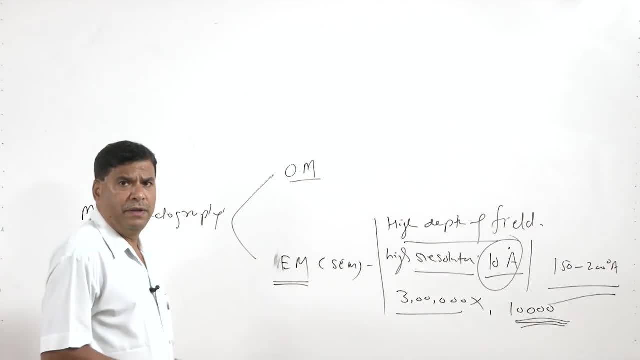 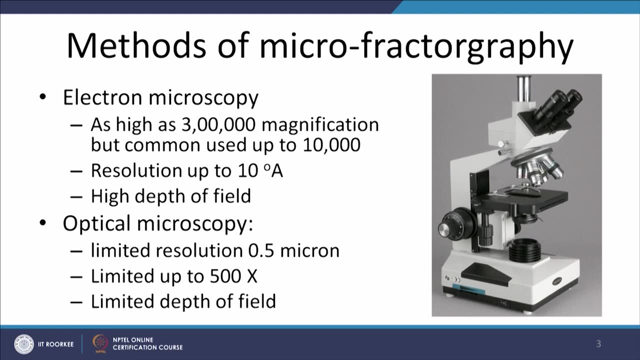 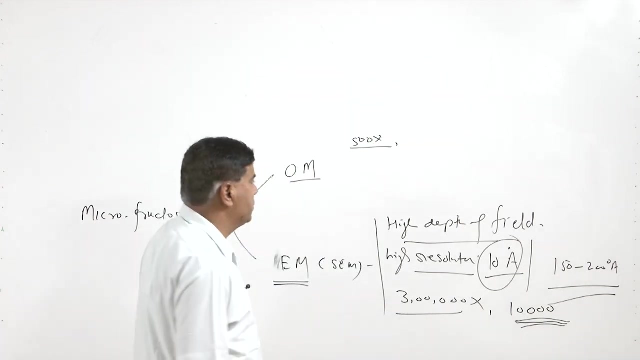 range also. So although we have the microscopes of the higher range also, where like 400 to 1600 magnification, but it is common that 500 X is the maximum magnification which is used and the resolution is also very limited, So we can say limited. 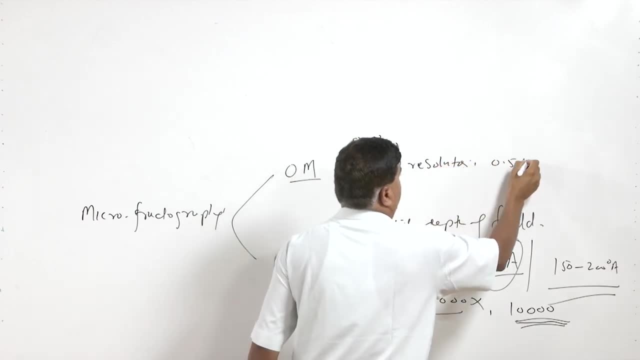 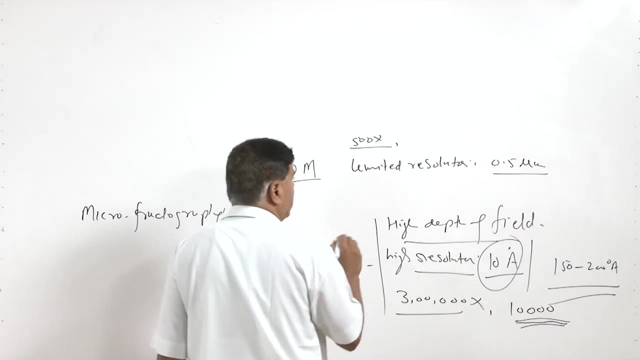 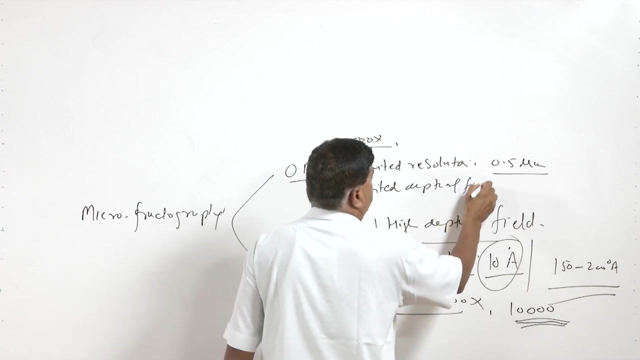 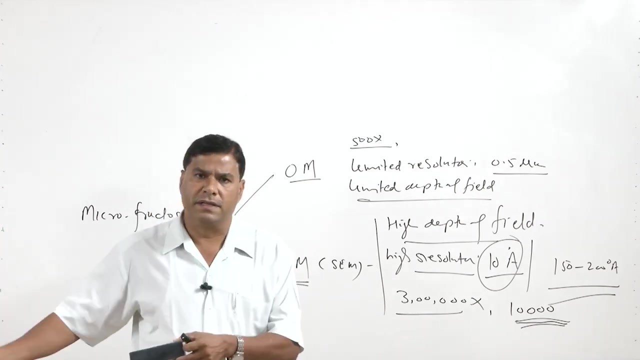 So limited resolution of 0.5 micrometer is available with optical microscopy. but another problem is the limited depth of field and because of this we may come across the problem where in one region is in focus and another region is out of focus, so lack of clarity. 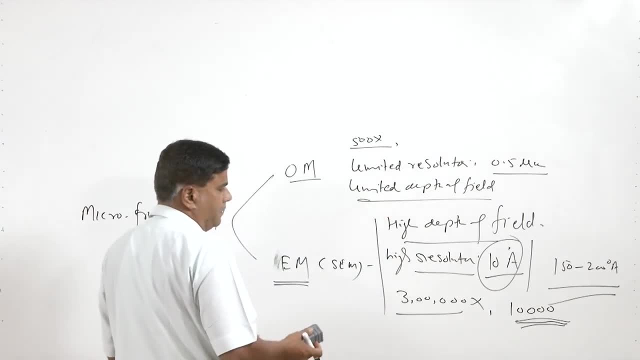 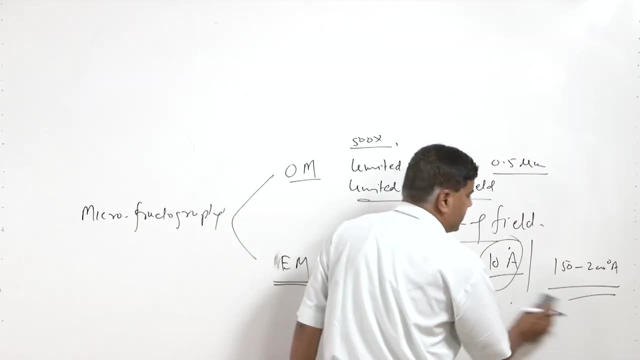 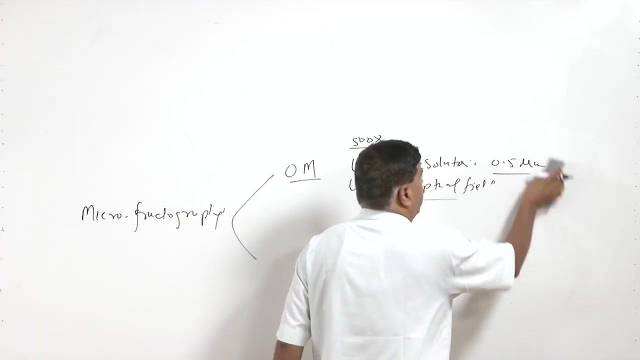 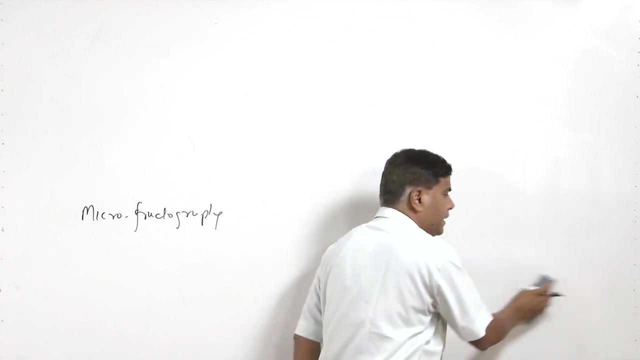 may be there in terms of the, The clarity on the microscopic features which are present on the fracture surface, and especially when these are seen at a high magnification. So these are the two tools which are commonly used for microscopy of the fracture surface, and thereafter we have the preparation of the fracture surface. how we can undertake 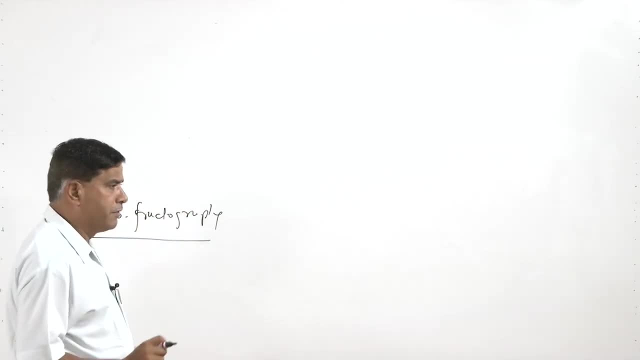 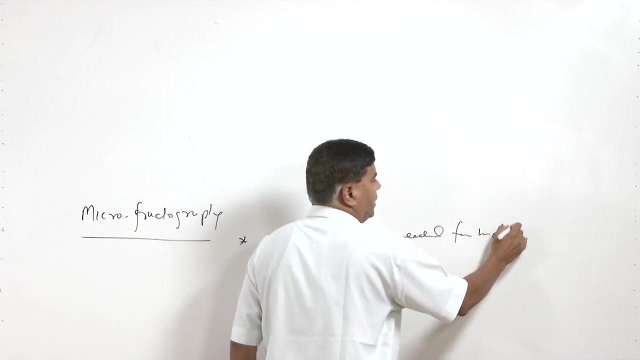 this. So we have the micro-fractography of any component. So mostly in case of the metals, no preparation is needed for metals because they are good electrical conducting, and for microscopy it is required that the surface of the workpiece is charged. 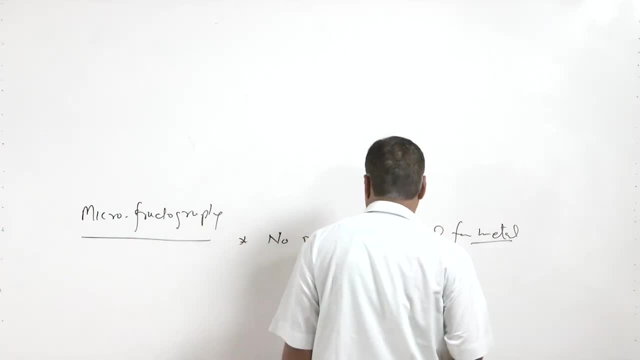 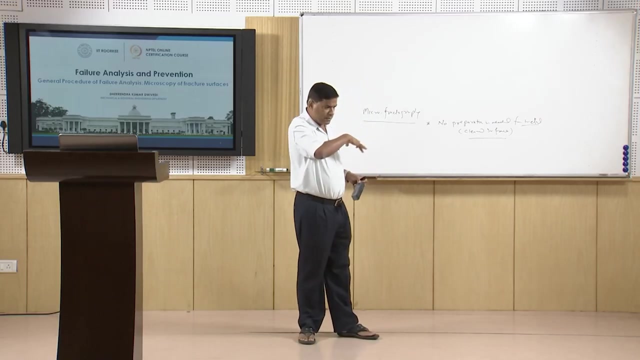 And the electron can be directed on to the surface of the fracture for capturing the, the images. But of course a little bit cleaned the surface which is to be observed is needed. So now with the fracture surface: if no oil, dust, dirt, grease, etcetera is present on 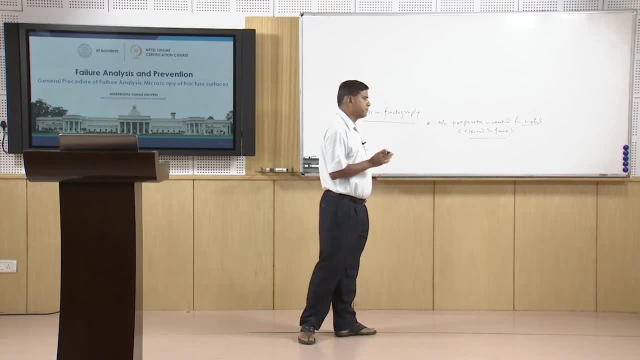 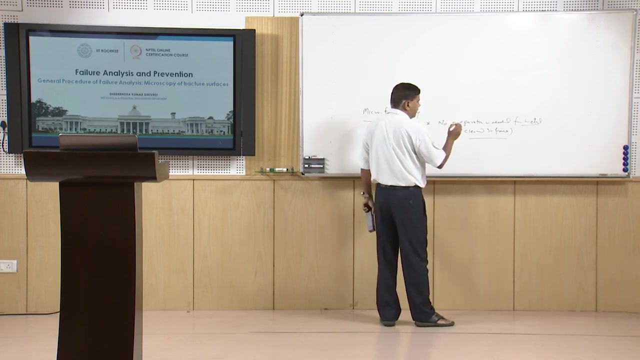 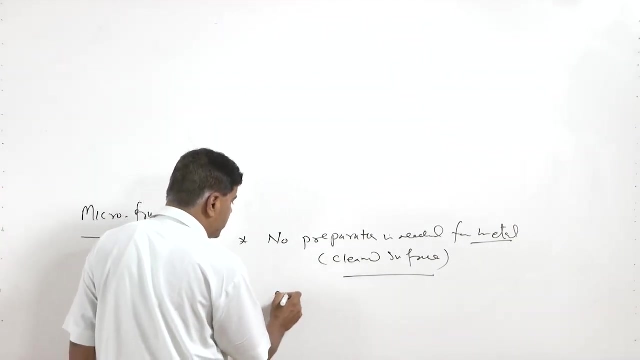 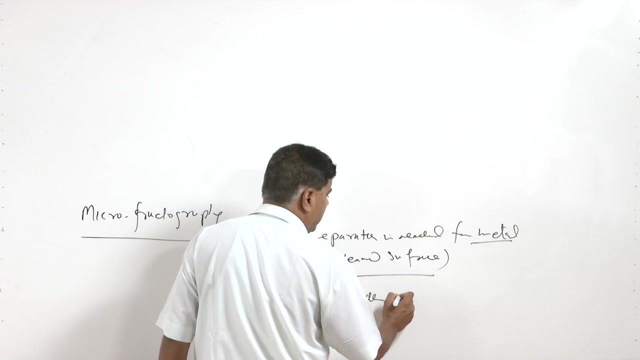 the fracture surface, then it can be easily observed. no special preparation is required. But of course, if these are present, then we need to clean the fracture surface in order to see the things, see the microscopic fracture mechanisms. So cleaning may be required if it is dirty, but in case of the powders or in case of oxides, 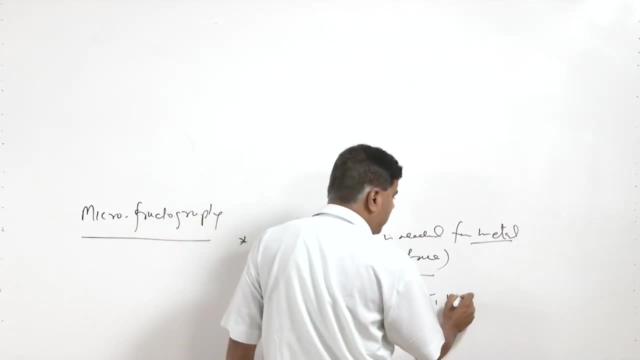 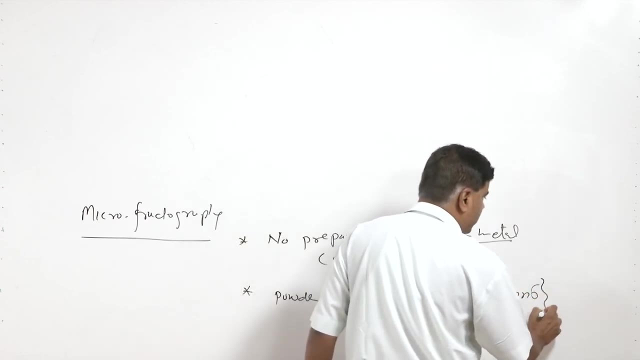 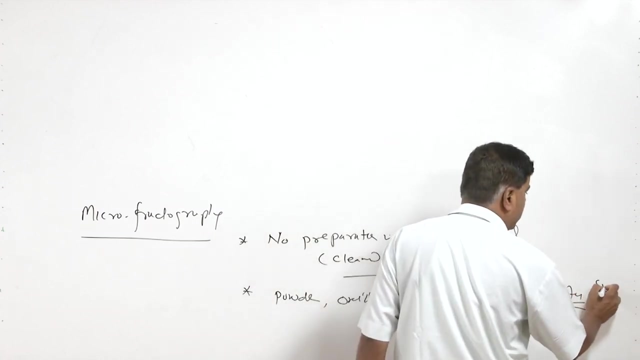 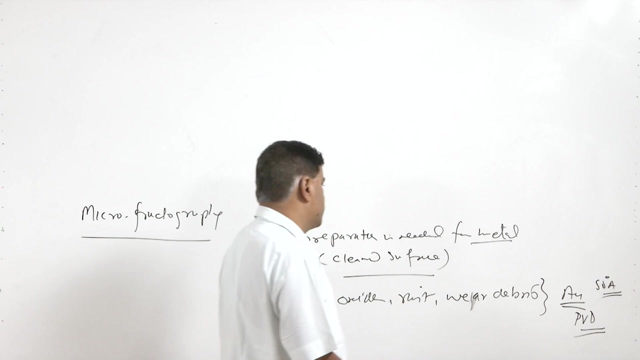 like rust or the wear, Wear, debris, it is required to provide the gold coating, coating of the gold which is, of, like, say, 50 angstrom thickness, and this is applied through the physical vapour deposition technique. So, in order to make the electrical conducting, as well as providing the good reflective surfaces, 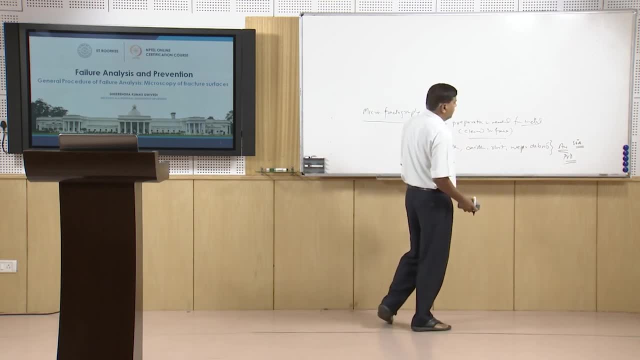 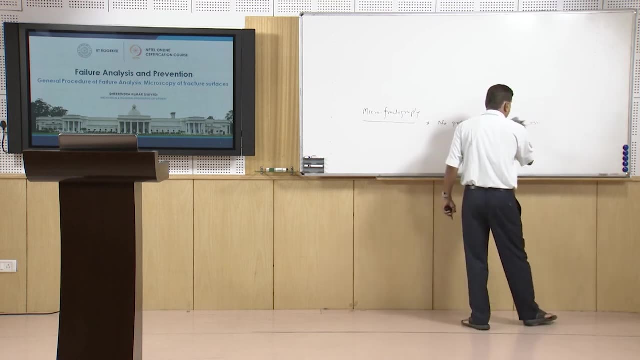 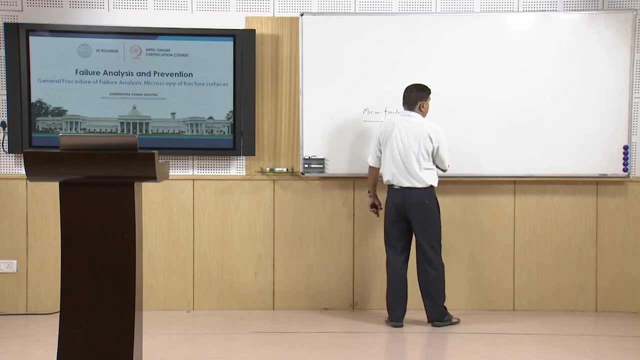 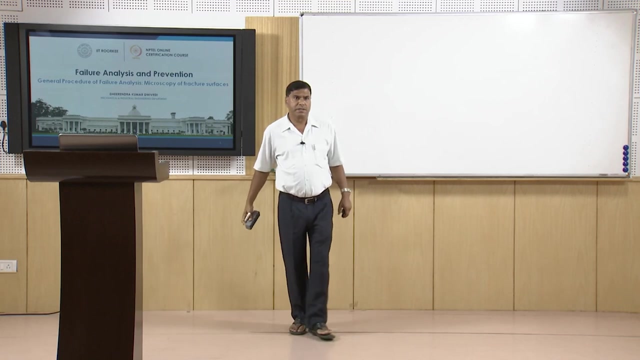 it is required that The non-conducting surfaces, if they are to be observed under the electron microscope, then these need to be coated with the gold of very using coating. thickness may be very thin just to make it electrically conducting and good reflection for the electrons. 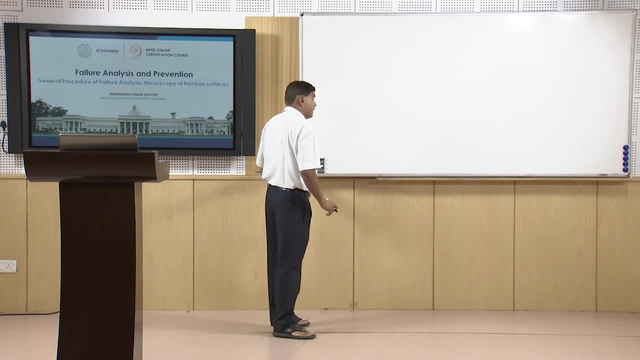 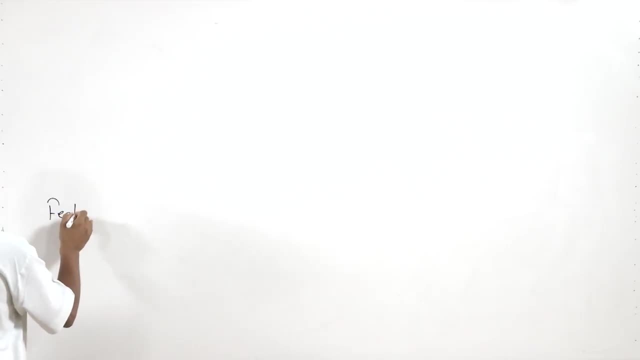 Then coming to the other microscopic fracture features. So they are basically the features of the microfractography. So there are four very standard microscopic features of the fracture surfaces and these are, like The dimples and the cleavage facets, intergranular fractures, features and striations. we will 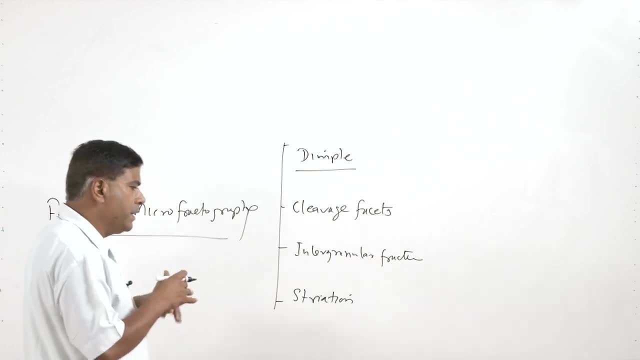 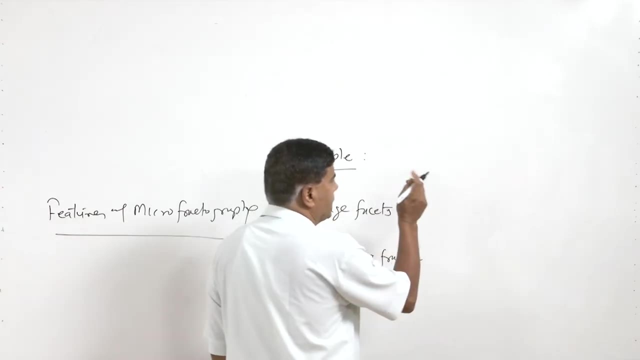 try to talk about what these indicate And when these kind of the features are observed. so the dimples are basically. these dimples are conical shaped features wherein mostly the inclusion or impurity which is nucleating the void is found at the bottom of the dimple. 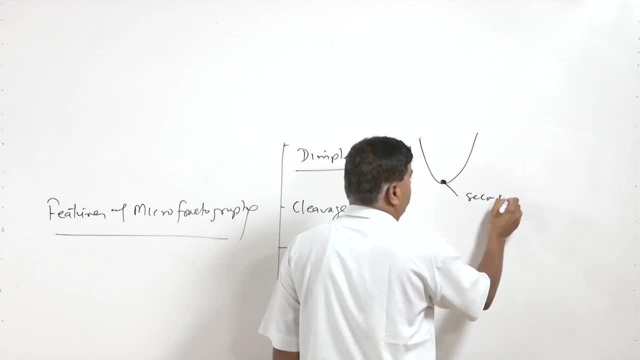 So this is basically the second phase. So the dimples are the particles, which is comparatively harder than the metal matrix. So this nucleates the voids and thereafter the metal matrix is subjected to the continuous deformation and it leads to the formation of the dimple kind of the features. 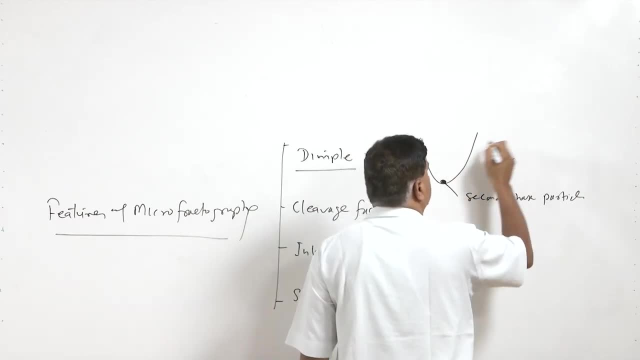 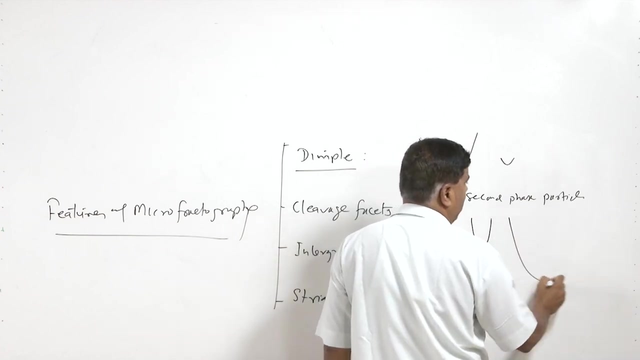 So the dimples may be shallow, like this, or these dimples may be very wide. So, depending upon the diameter of the dimples, like this, this is a conical shape, So the dimples may be of a smaller diameter or the large diameter. 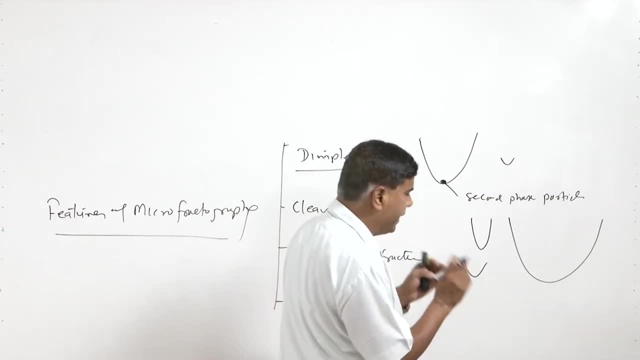 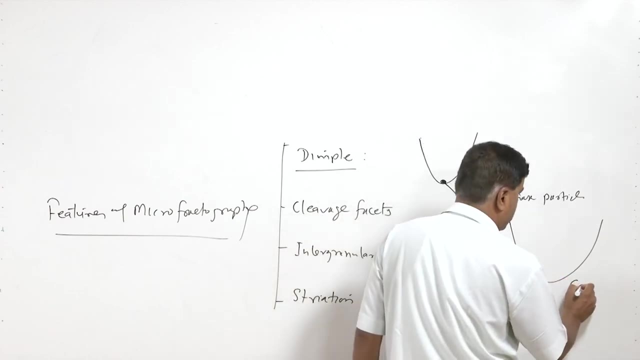 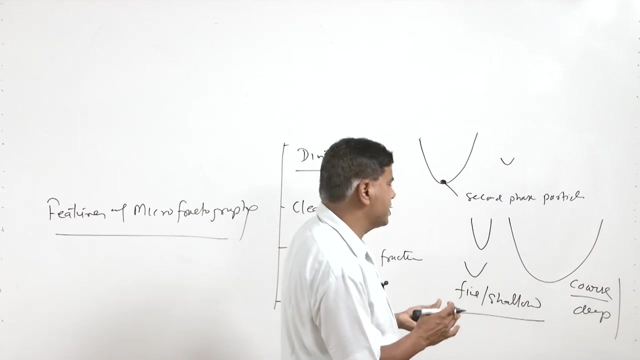 Dimple may be shallow or fine. So basically fine and shallow dimple, or it is a coarse or very deep dimple. So if the coarse and deep dimples is there, then it will indicate very extensive plastic deformation compared to the case when the dimples are fine and they are shallow. 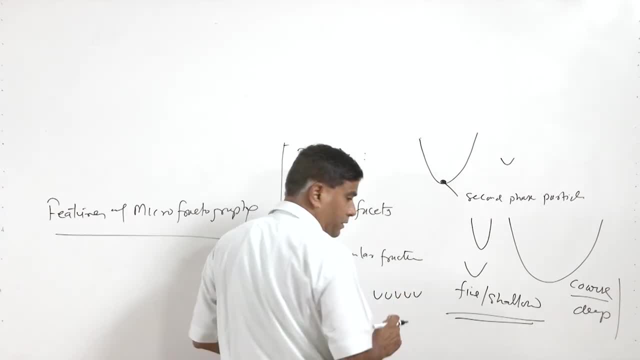 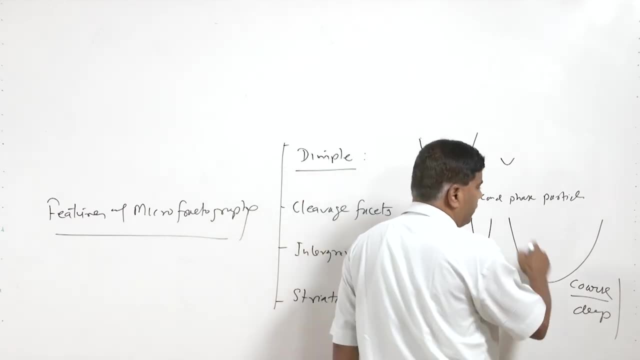 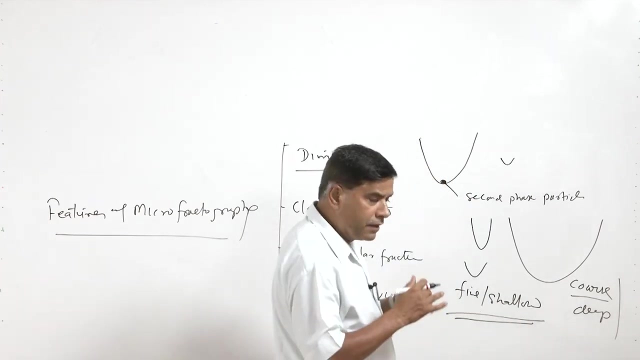 Large number of the fine dimples indicates the possibility of the good yield strength of the material, but the limited deformation. On the other hand, extensive deformation and the large or coarse dimples indicate somewhat lower yield strength and the greater ductility or the percentage deformation prior to the 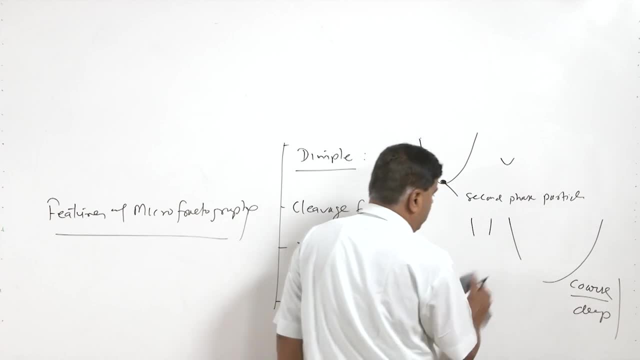 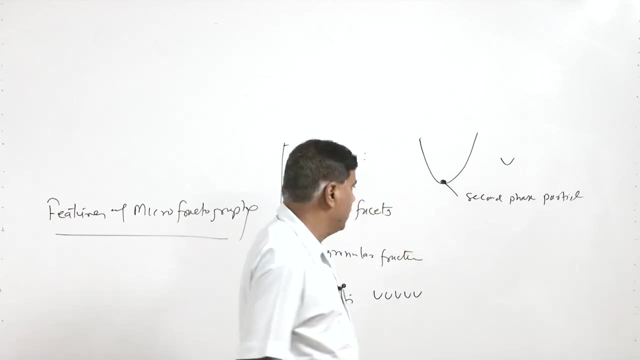 fracture. So the percentage elongation and the fracture would be more in case when the dimples are the large and the depth is more as compared to the case when they are fine. So the dimples, these are basically formed when the material which is filling is ductile. 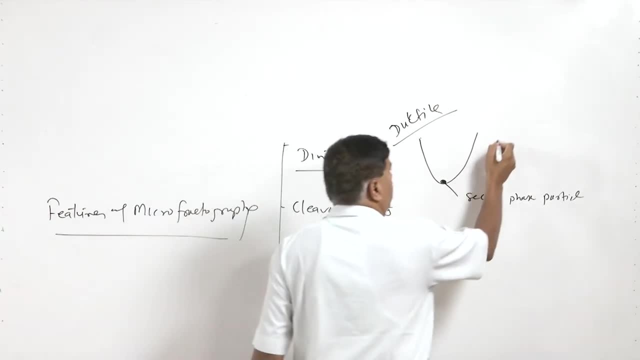 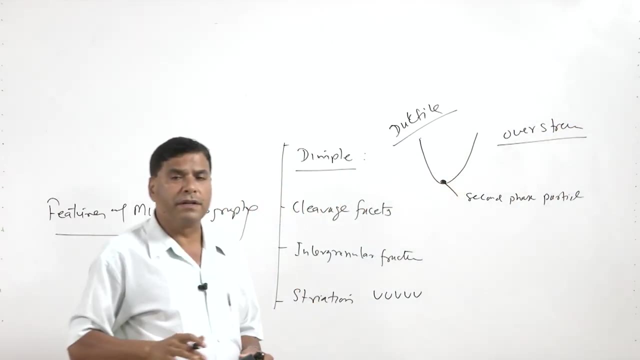 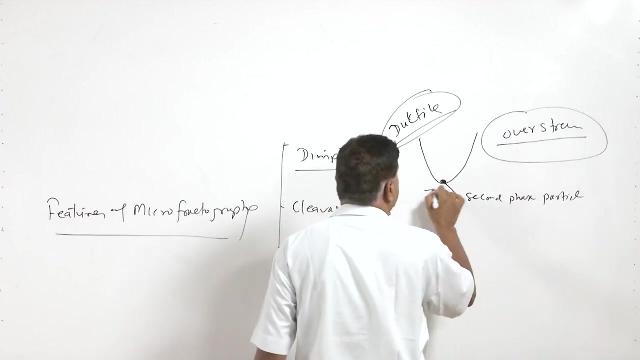 and this kind of the fracture is observed under the over stress. So this means the component has been subjected to the overloading. So the ductile metals subjected to the overloading will indicate the dimples. This is very common understanding. when the dimples are shallow and the fine the loading. 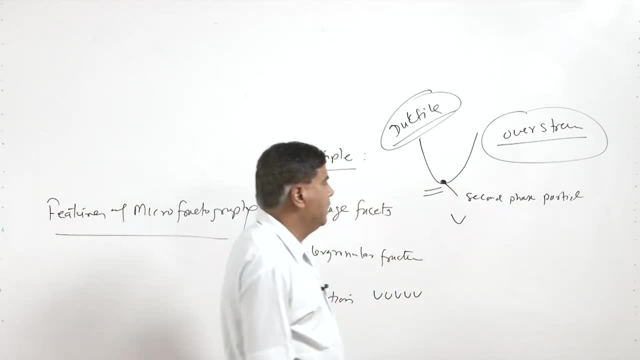 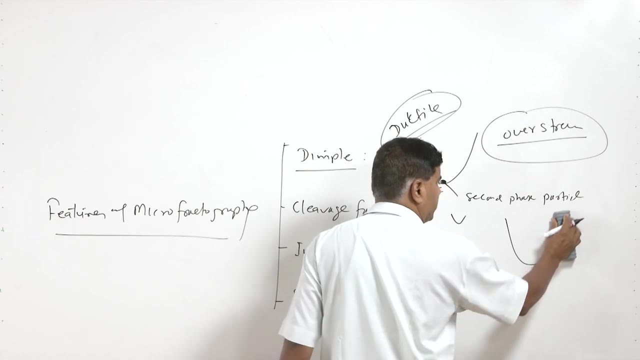 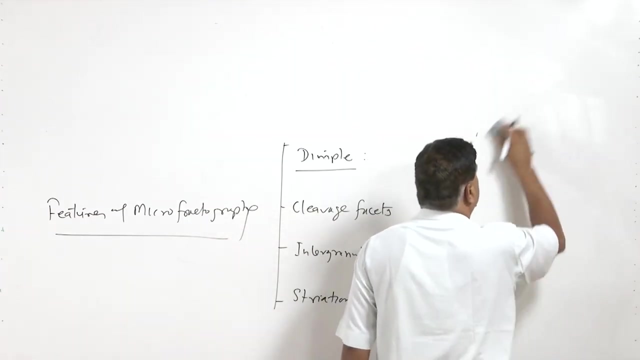 capacity is high, but the ability to deform is limited, while when dimples are large, coarse and deep, Then yield strength will be low, Ductility will be high. So these are the kind of inferences about their ability to carry the load and the energy. 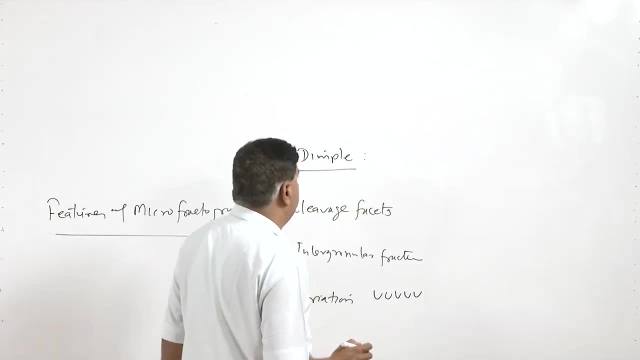 required to cause the fracture. There is one thing which is common: that whenever the dimples are observed, dimples are considered to be high energy fracture. Whenever dimples are present onto the fracture surface, it is considered that it would have 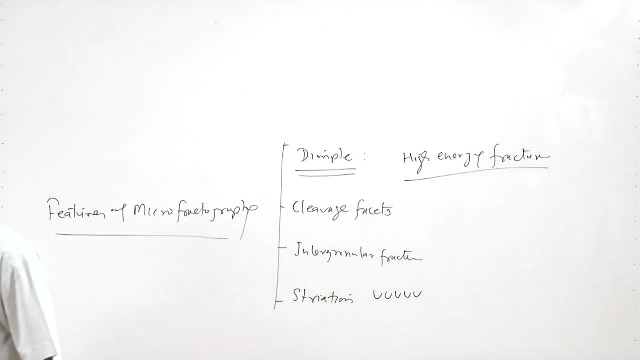 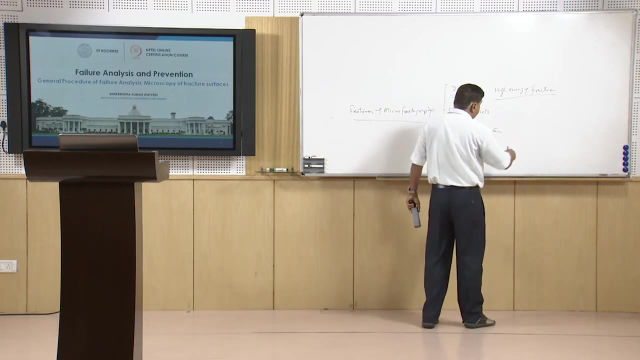 a it would have needed. So it is considered to be high energy fracture. So it is considered to be very high energy for causing the fracture There, while the presence of other features will indicate the possibility of the low energy fracture. We will be talking about that now. 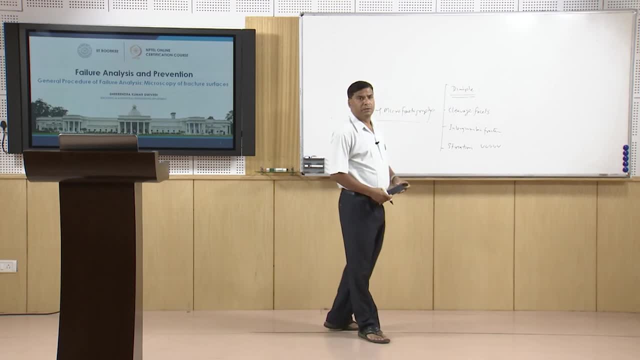 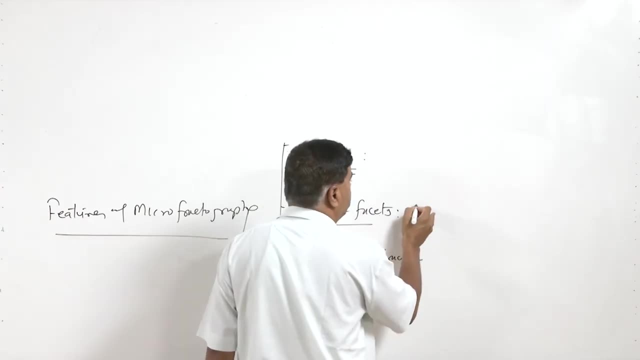 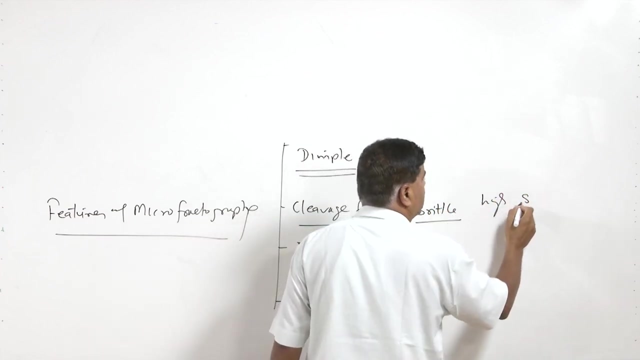 So the cleavage facets. now, the cleavage facets are the another general microscopic features which are normally observed when the material is low. The material is the brittle in nature. So in metals like high carbon steels, high carbon steels, which show limited ductility. 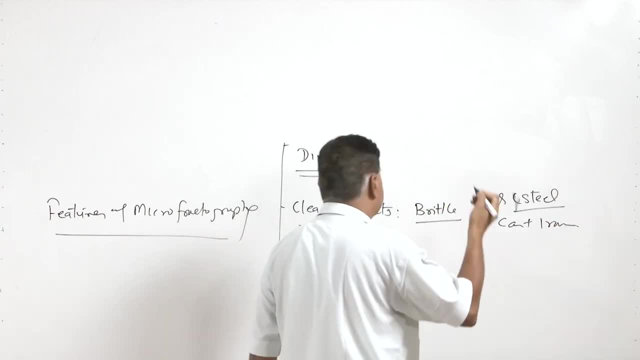 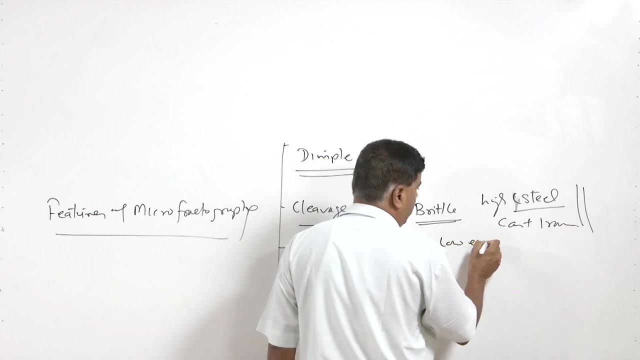 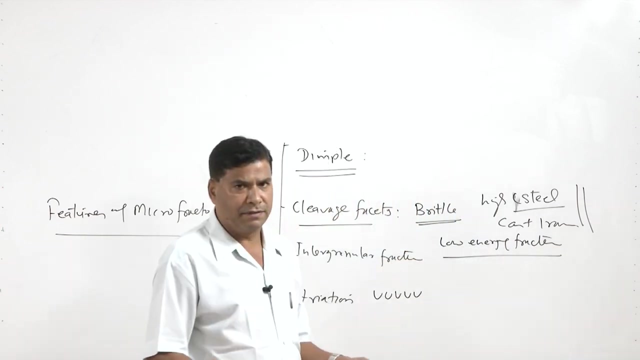 cast iron and other high strength metals which show very limited ductility. they tend to fail in brittle manner. So the cleavage facets is one of the indicator of the low energy fracture And whenever it is present, material is said to be of the low fracture toughness it will. 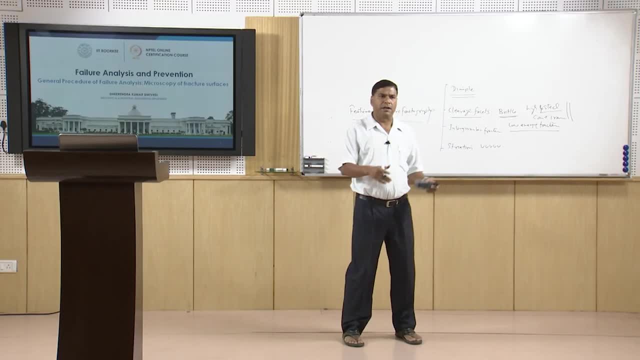 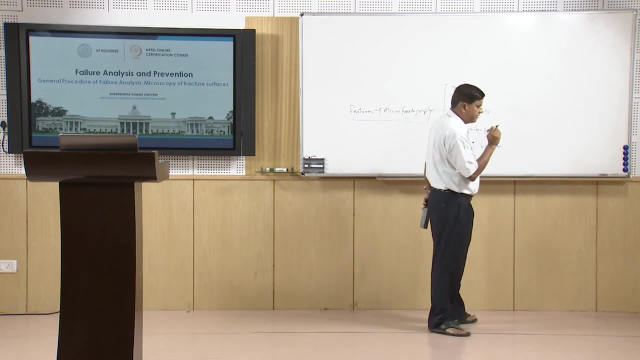 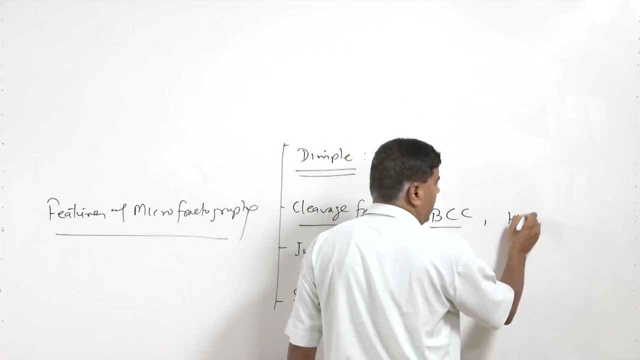 require less energy to cause the fracture as compared to the case when the where the dimples are present onto the fracture surface. And this kind of the feature is observed normally in case of the BCC metals and the HCP metals, but not necessarily. 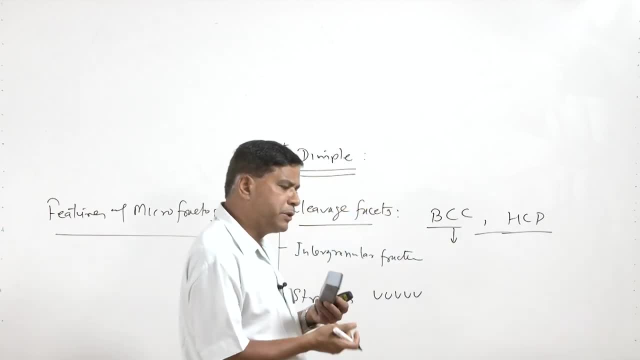 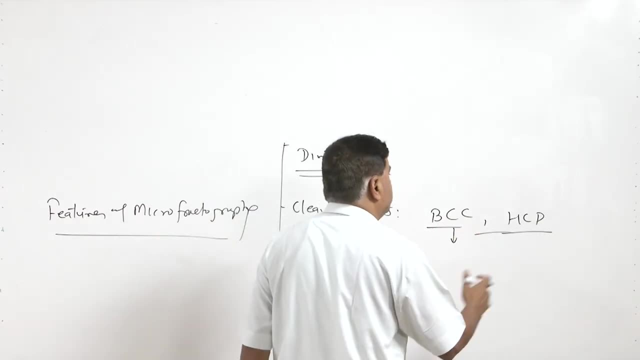 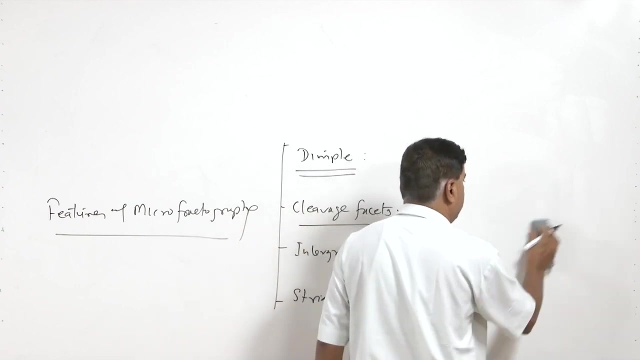 Because the iron, if it is pure, it will show lot of elongation, like 30-40 percent, and with lot of ductility. but certain compositions of these metals indicate very limited ductility and the fracture in those cases is mostly through the cleavage facets mechanisms. 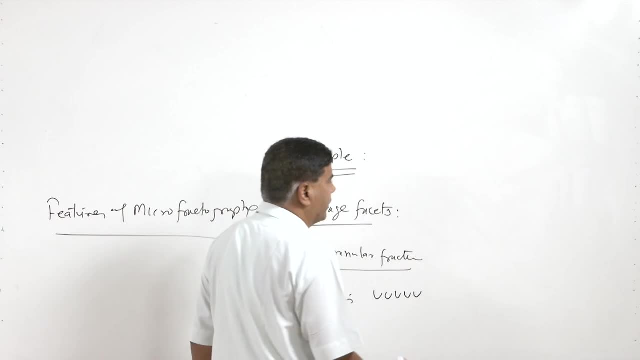 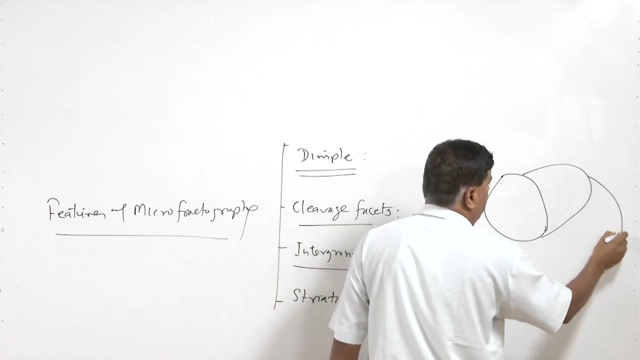 Intra granular fracture. intra granular fracture is the typical one where the crack, if it is present, That will be propagating through the grain boundaries, So like in a metal system. these are the number of grains present on to the fracture surface. 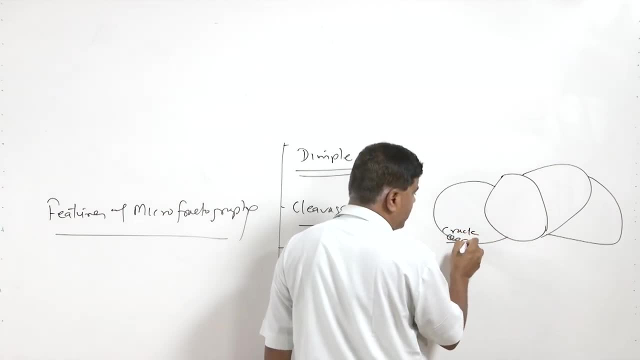 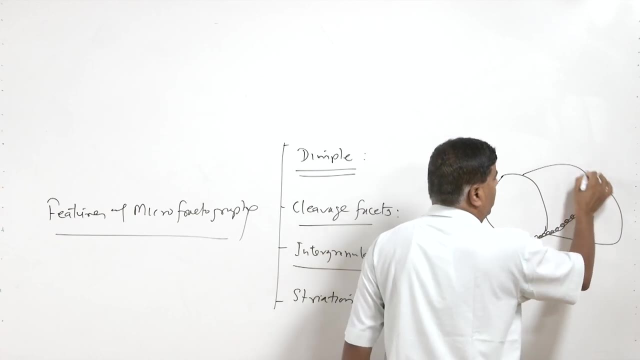 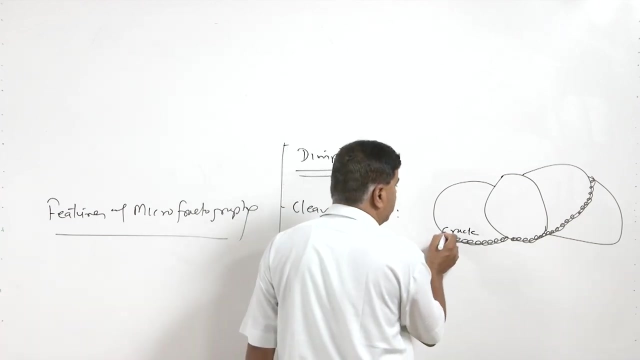 So sometimes the presence of the poor phases at the grain boundary, or undesirable, precipitates in form of the plates or in form of the flat, in form of like thin layer. So in case of the poor phases, which are brittle, have limited load carrying capability or like. 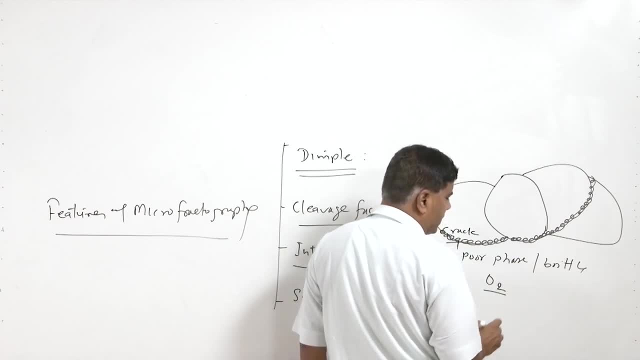 precipitation of undesirable constituents like oxygen in case of the nickel alloys. So these provide very low strength, low ductility zones where which, under the favorable conditions, if the crack Crack has nucleated, then it will easily propagate through these grain boundaries. So the propagation of the crack along the grain boundary will be leading to the inter. 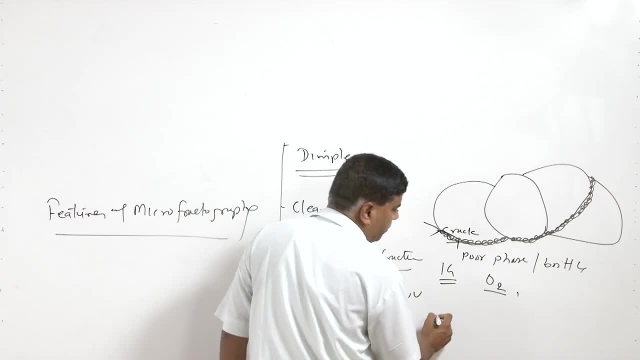 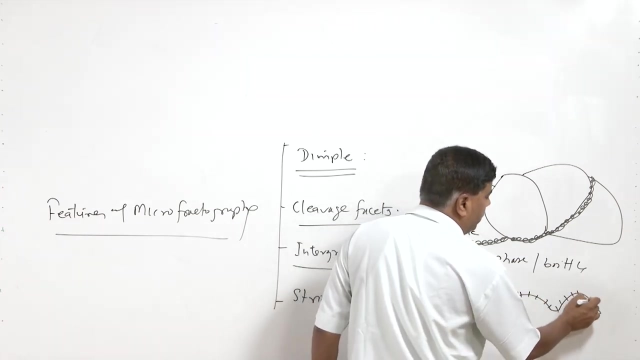 granular fracture and whenever it happens, what we will find? that fracture has a separated fracture. the separation of the grains have taken place through the grain boundaries and in that case The grain boundaries So will be exposed to the surface in this form. So we will be able to see that different ball shape constituents are present on to the fracture. 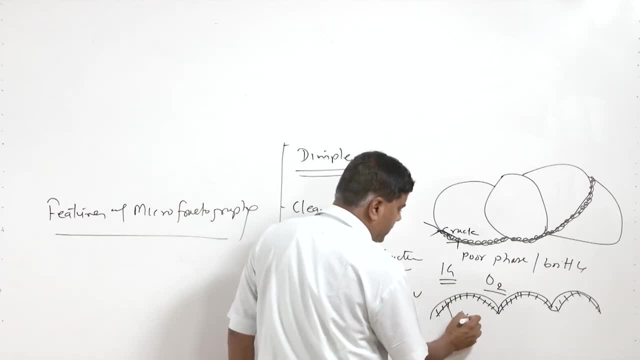 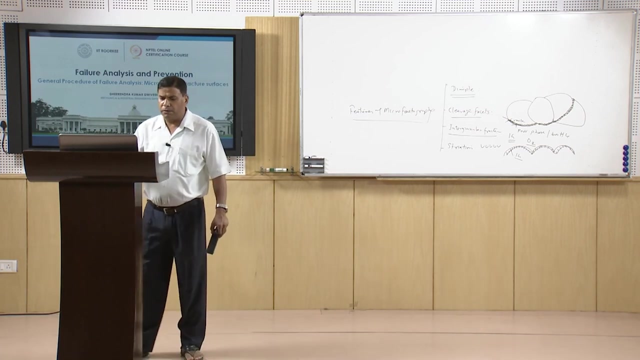 surface, indicating that fracture has taken place in inter granular manner. So this is what we can see here: that the brittle inter granular fracture, whenever it occurs, the different grains will be clearly visible on to the fracture surfaces- And which is indicating that the crack has propagated along the grain boundary and the 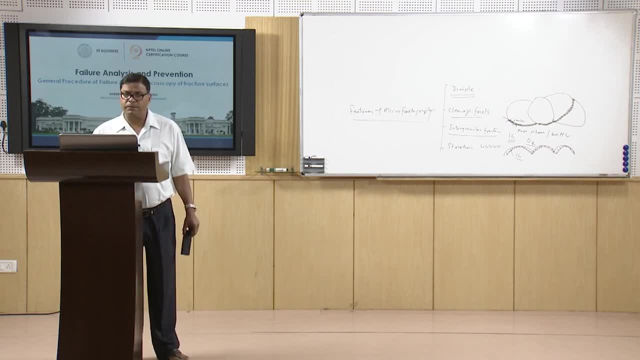 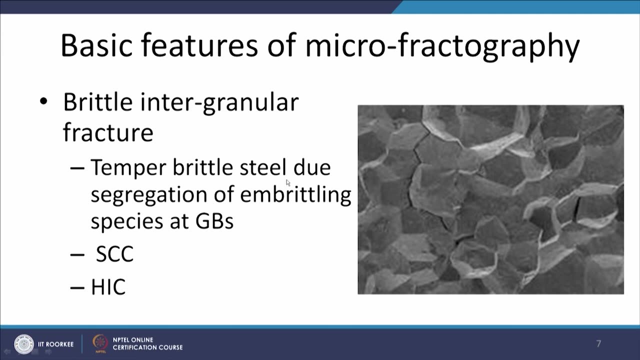 separation of the grains have taken place through the grain boundary And this kind of the fracture is observed, like, say, in case of the tamper. brittle steel, due to the segregation of the embrittling species, is at the grain boundaries. This kind of fracture is also observed in case of the stress, corrosion, cracking and 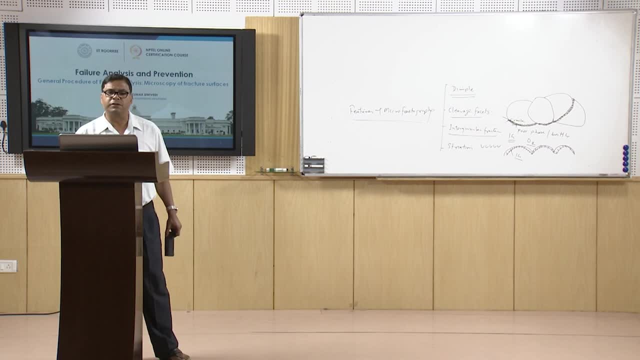 the hydrogen induced cracking. So this is what we know is at first. So this feature is indicative of the brittle fracture due to the growth of the crack through the grain boundaries, leading to the exposure of the grains at the fracture surface, and so this is basically brittle intra granular fracture. 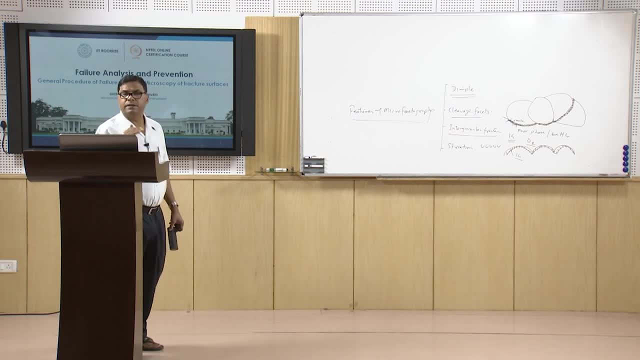 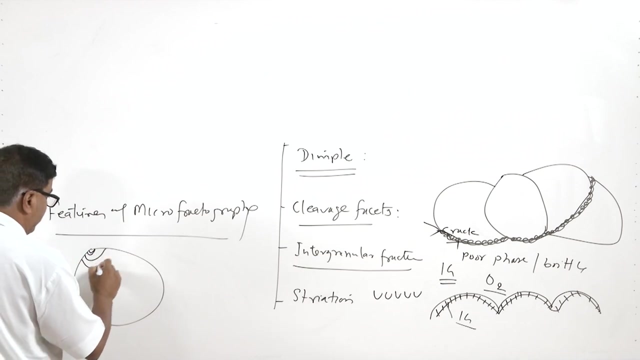 And the fourth feature is it is the striations, as I have explained earlier, whenever, during the fatigue fracture, first of all the nucleation of the crack takes place and thereafter the crack will be growing in a particular direction. in case of the unidirectional loading, 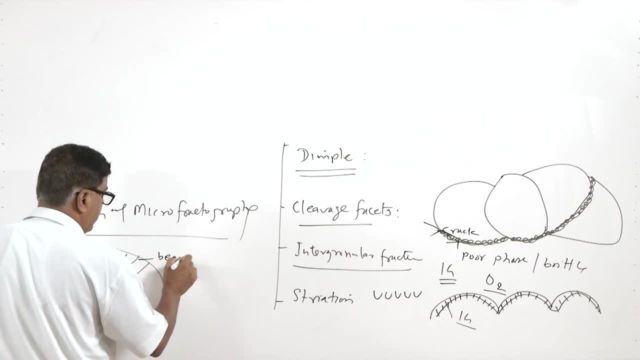 So this will be leading to the presence of the beach marks, which are the concentric circles having the center at the location of the crack initiation, and thereafter it experiences the sudden fracture which is basically overload fracture. Overload fracture may occur through the dimple or through the cleavage facets. crack growth. 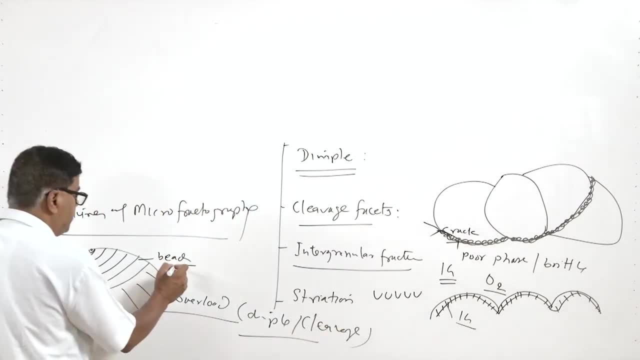 mechanisms and these beach marks at high magnification appears in form of striations, which indicate the magnitude by which the crack is growing under the each load cycle. This is the theoretical one, but actually it requires lot of load cycles for growth of the crack. 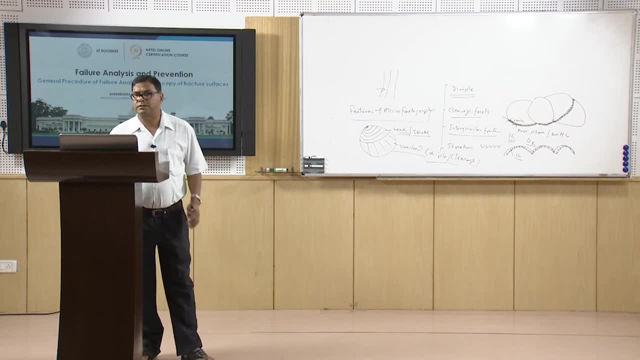 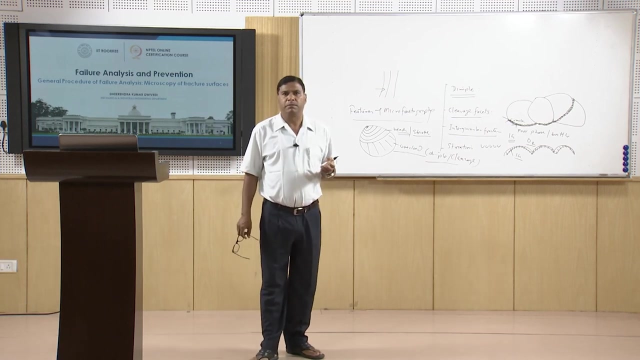 So whenever the striations are present on the fracture surface, it indicates that the load has been the cyclic in nature and the fracture has occurred in fatigue manner. Now I will summarize this presentation. In this presentation I have talked about the purpose of the microfractography and what 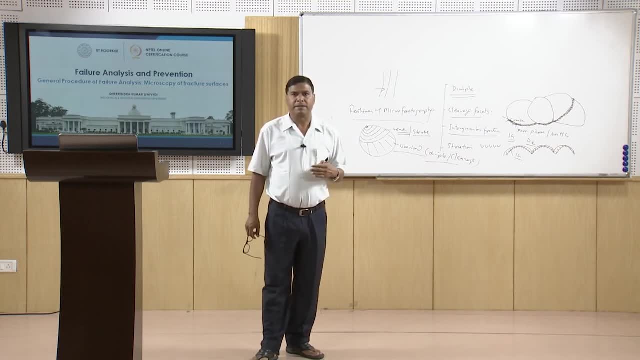 are the general microscopic fracture mechanisms or the features And which can be used to interpret the kind of the way by which fracture has taken place and the kind of loading conditions which were experienced by the component during the fracture. Thank you for your attention.